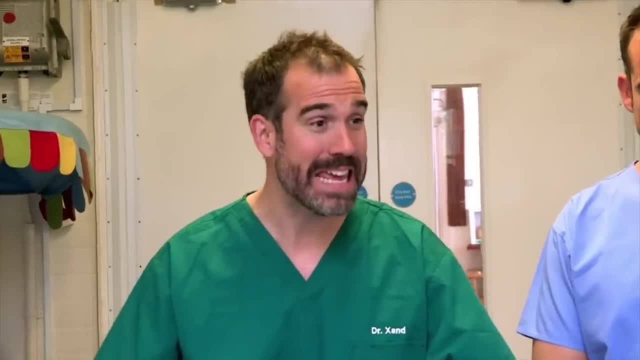 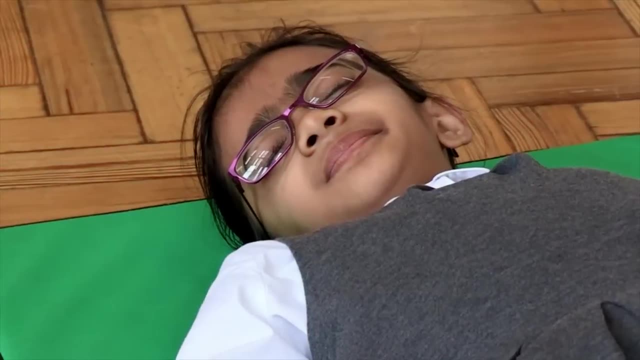 But will this lot get it right with no training? Are you ready? Yes, Off you go. Ajay and Hanitha are both pretending that they've had an accident and are unresponsive and not breathing. Quick guys, they need your help. 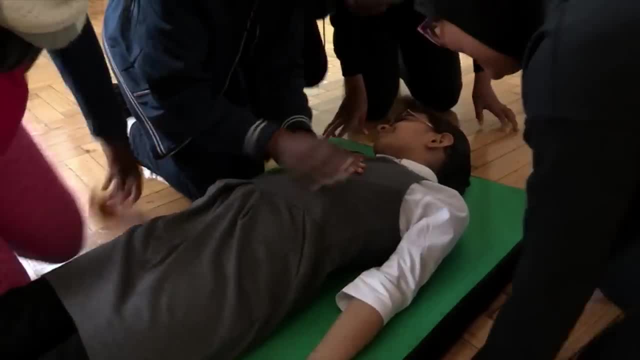 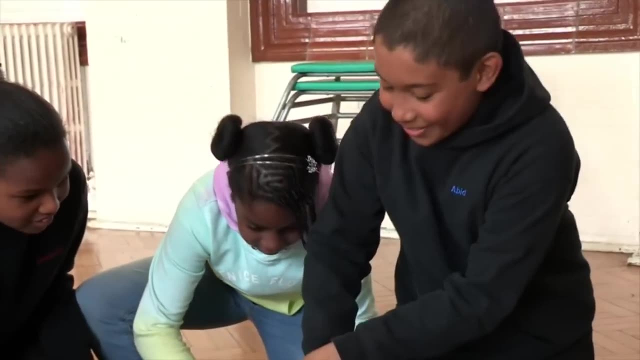 I want food. Okay, you got a phone. No, no, no, You need to come to this location straight away. Or calling an ambulance is a great start. I can't feel it. Start the compressions one. They've got into doing chest compressions but actually they're just squishing his stomach. 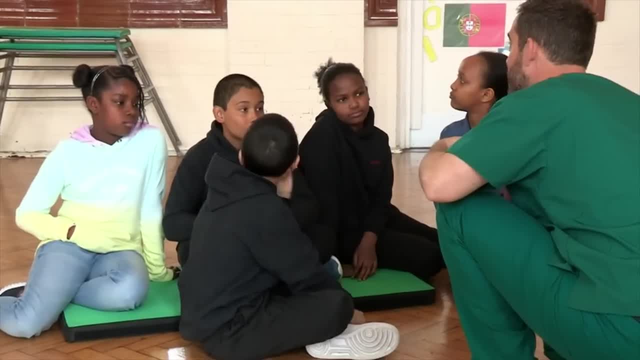 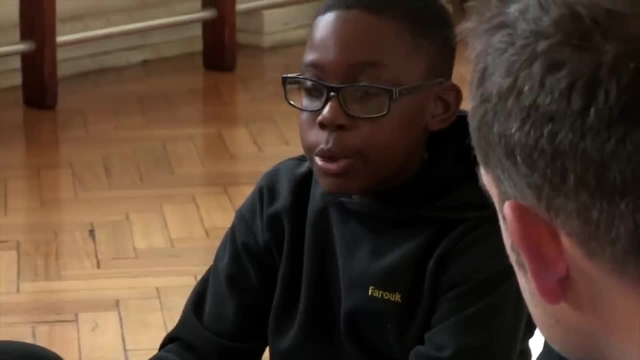 They're not doing them in the right place at all. Our teams didn't quite get this right. Some ideas were spot on, like Farouk's. I searched to see if she had a phone on her so we could call the ambulance. 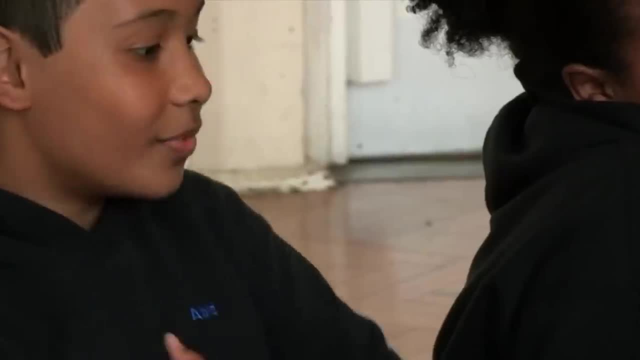 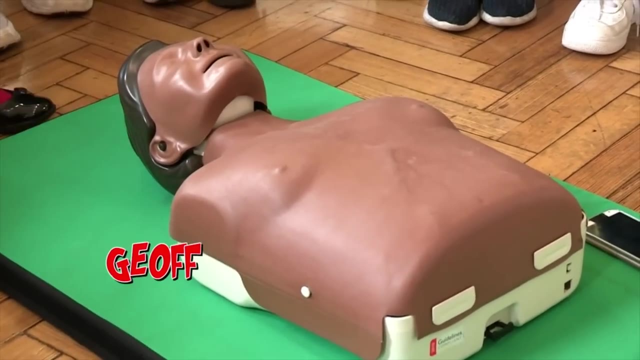 Others just missed the mark. Tell me about the chest compressions. I don't think I did it too next to his chest. I was doing it near his stomach. Let's show you how it should be done with the help of Geoff. Off you go. 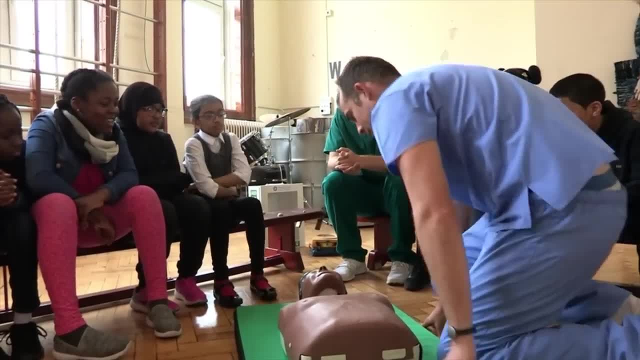 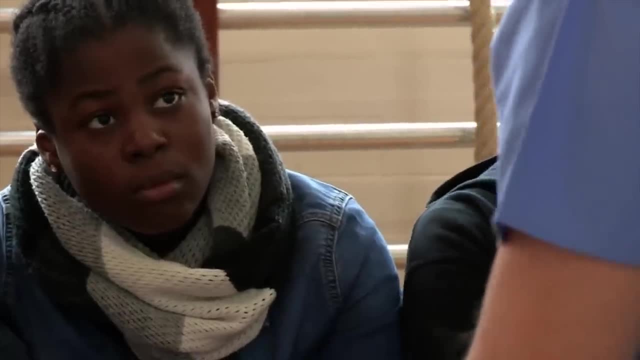 Our first aid dummy Right. can you see if he's responsive? Geoff, Remember, we're showing you what to do in an emergency, but it's always best to get an adult. I'm shaking him gently, but he's not saying anything. What should I do next? 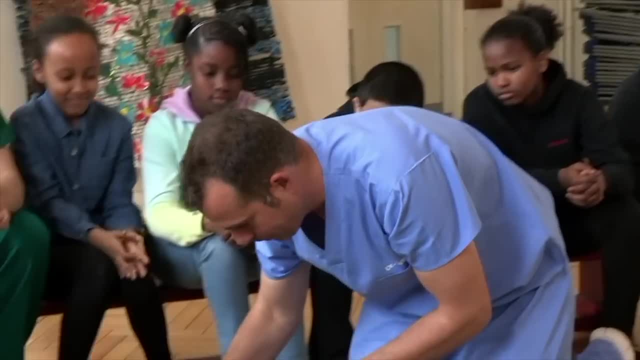 Can you check if he's breathing? Yep, Put your ear down next to his mouth. Tilt his head back. Can you feel any breaths at all on your ear? No, I can't feel any and I can't hear anything. 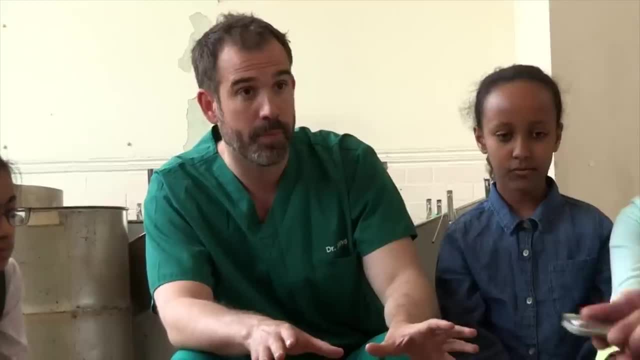 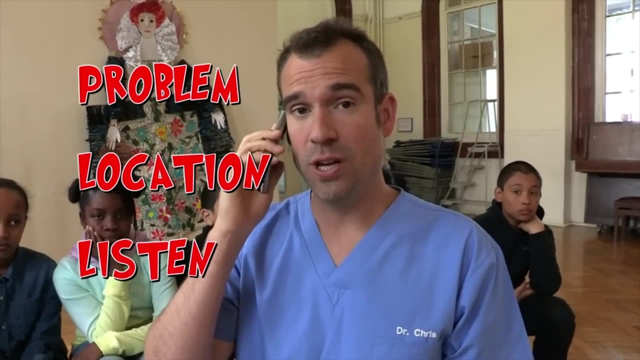 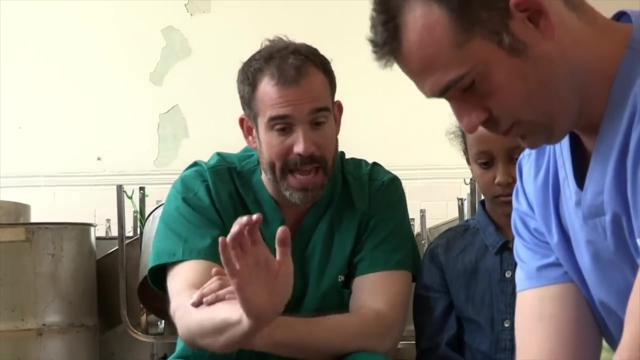 We need to call 999.. Okay, I've got a phone here, So you call 999, give the patient's problem, Give your location and the ambulance service will tell you to start doing chest compressions. Put the heel of your hand in the middle of his chest and start pushing down at that speed twice every second. 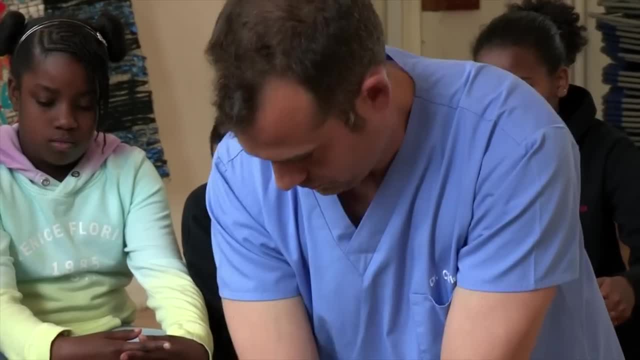 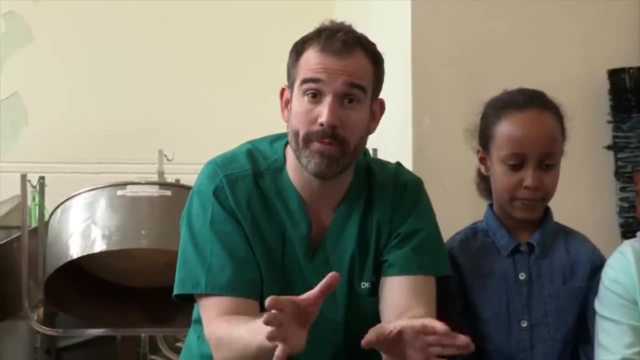 To do chest compressions you need a grown-up, because it's hard work and requires the stronger power of an adult for it to be effective. So Chris is now doing chest compressions. I need to go and find an AED or defibrillator. 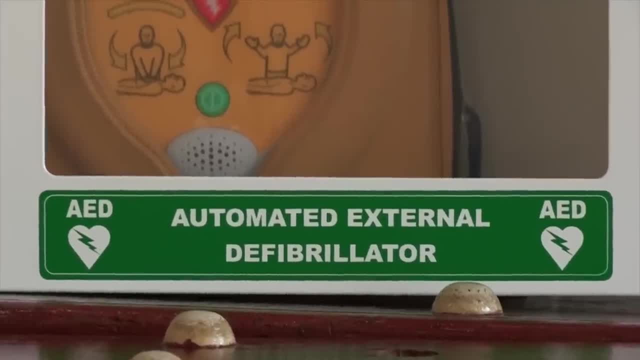 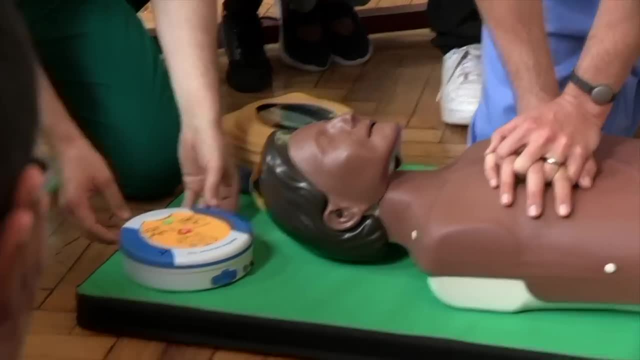 An AED or automated external defibrillator can be spotted in schools and public places like sports centres. Now all AEDs have instructions on them. It's a machine which delivers an electric shock to the heart. Pull green tab to remove pads. 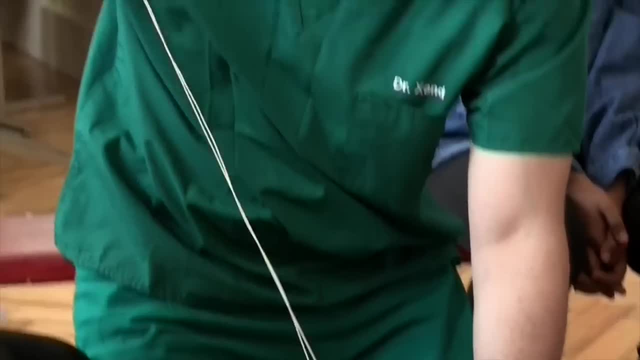 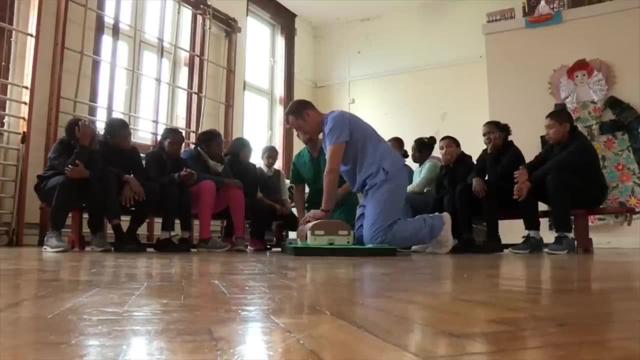 There are the pads: Peel pads from liner, Press pads firmly to patient's bare skin. Okay, and now you need to move back because I'm going to give a shock. Can you stand back? Geoff isn't responding because he's a dummy. 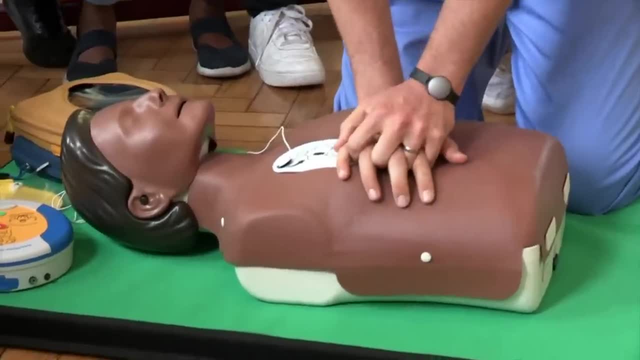 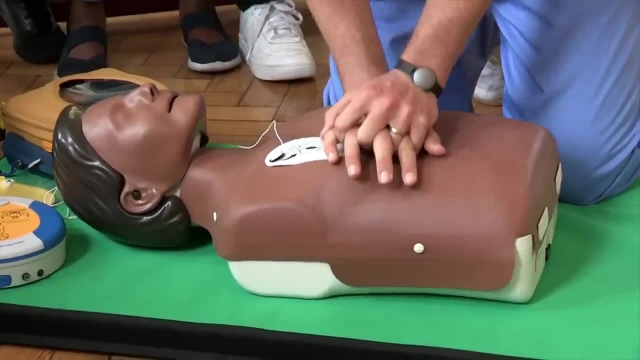 But at the touch of a button, the defibrillator tries to give the heart a kickstart. This machine will talk you through everything you need to do, so the most important thing is to stay calm and listen to the instructions. Do you want to have a go? 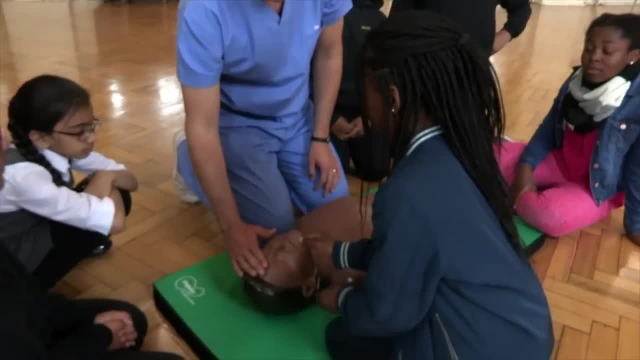 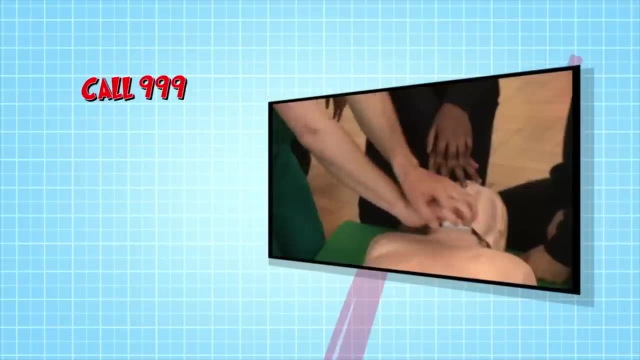 Yeah, Brilliant. So if you see someone who's unresponsive and not breathing, call 999.. Remember you'll need to know your location. Then tell an adult how to do chest compressions And finally, if available, find a defibrillator and follow its voice orders. 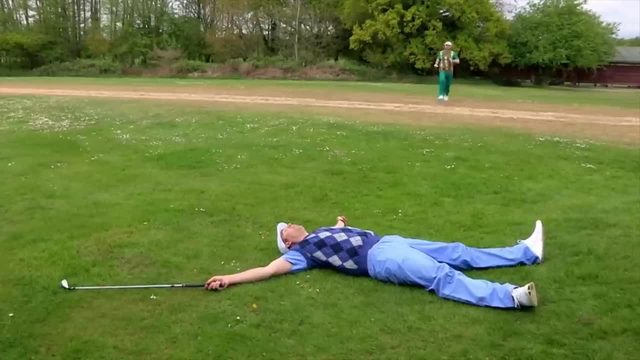 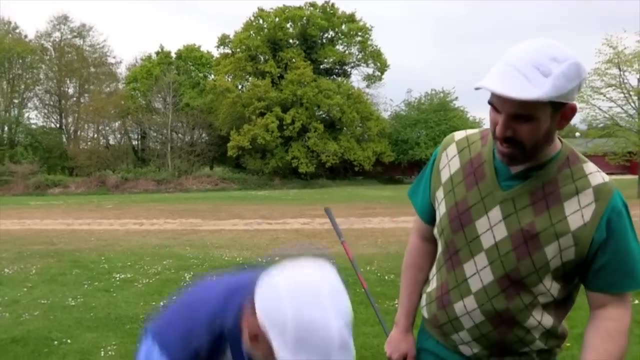 Good work guys. Chris, are you breathing? Oh, yes, I am. I just winded myself. You winded yourself, Is that it? Yes, but it was quite a shock at the time. I thought it was some kind of emergency. 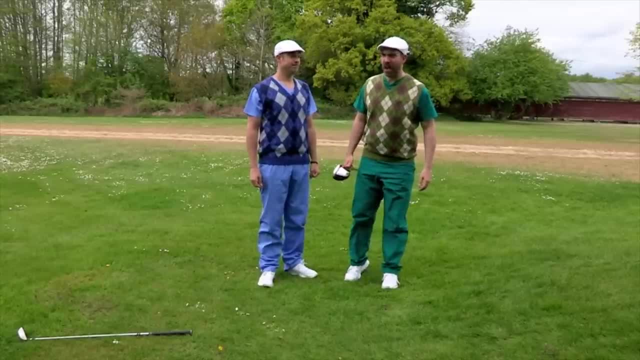 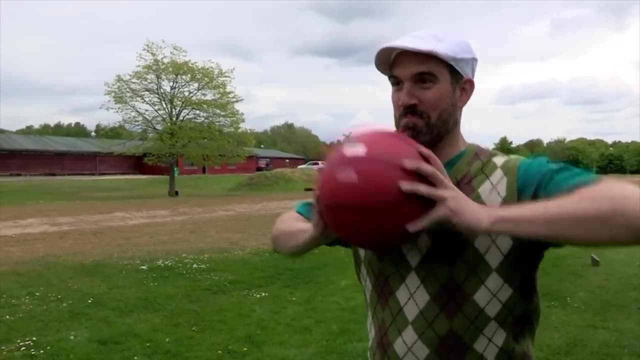 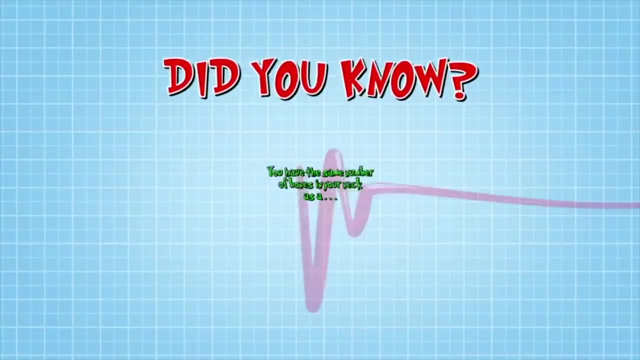 Well, it's always better to check. I wonder if we should play something else. I've got this basketball with me, Okay, all right, Ready. One, two, three, Winded again. Ouch, Did you know you have the same number of bones in your neck as a giraffe? 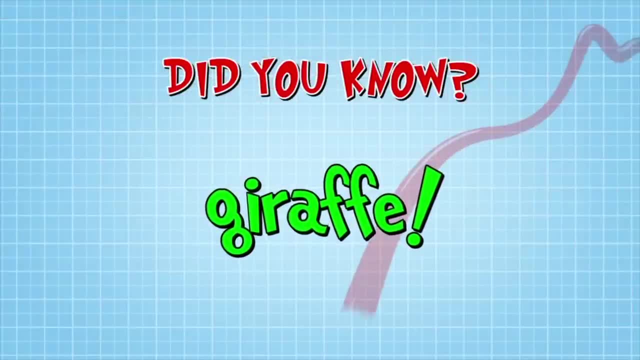 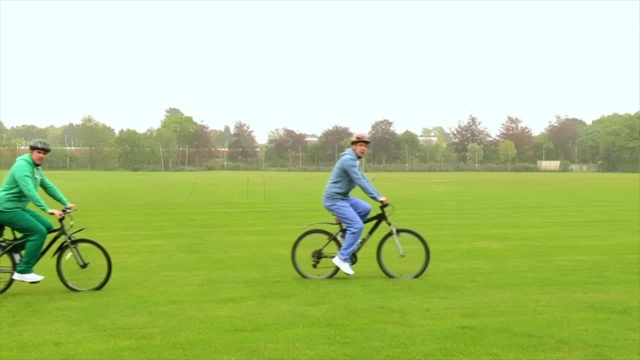 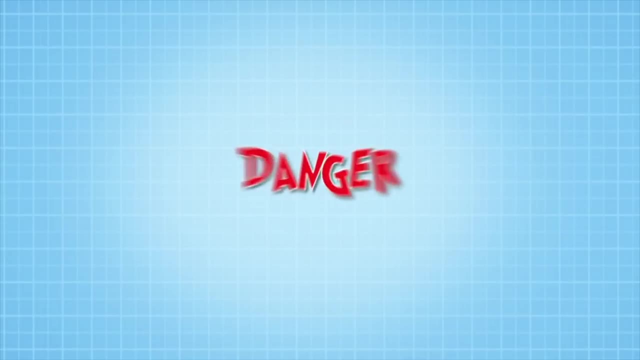 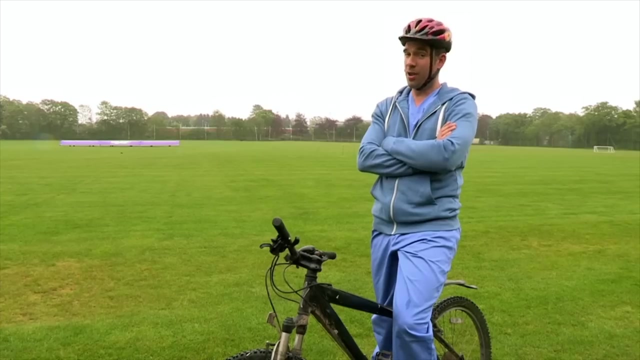 Those are just bigger, But all bones need looking after. Cycling in the park: Brilliant exercise and a brilliant way to get some sunshine. But of course, cycling can also be dangerous. You could cycle into a hedge and hit your head. That's why I'm wearing this snazzy helmet. 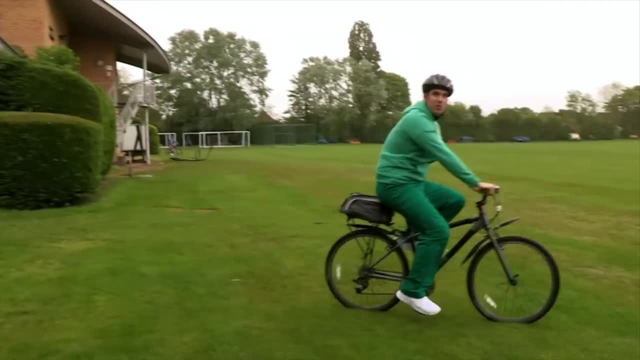 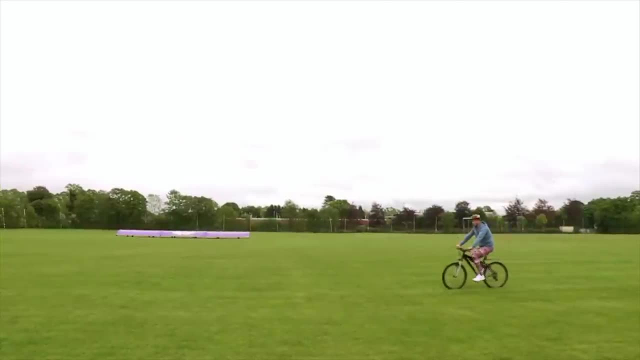 Or you could fall off and get a nasty graze on your knee. That's why I'm wearing these snazzy leggings. And finally, of course, you need to make sure your bike is properly maintained. You wouldn't want to squeeze your brakes and 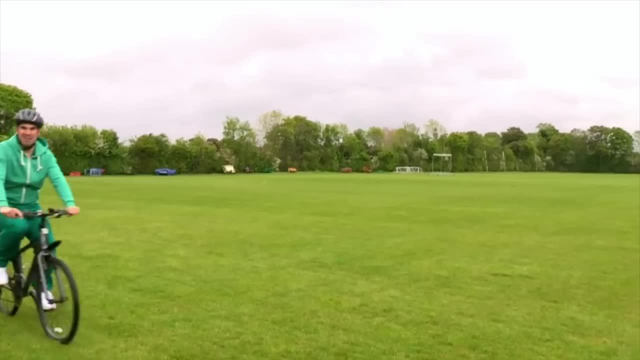 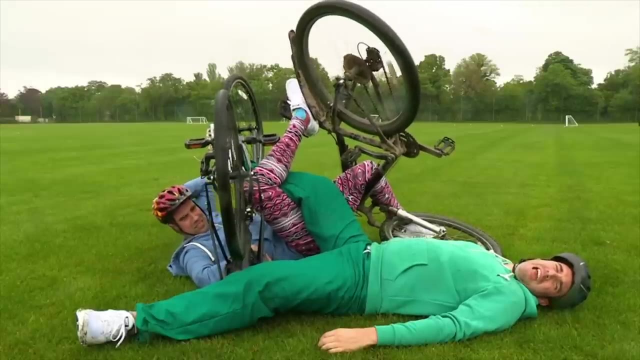 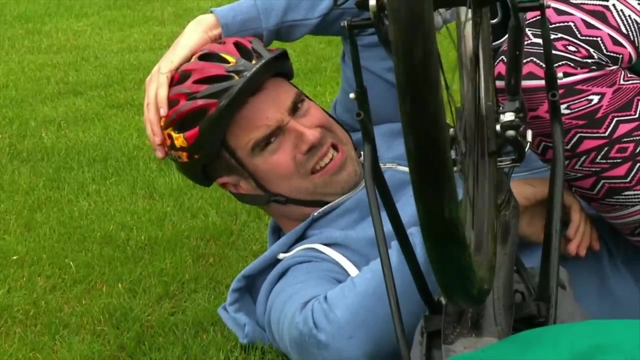 Uh-oh, my brakes, My brakes. Well, thanks for my helmet, Thanks for my helmet. I don't have a head injury, Me neither, and thanks to these leggings I haven't got any grazes, But on the downside, I think I've broken my arm. 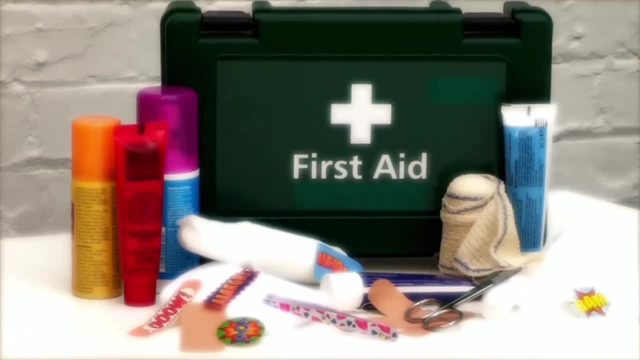 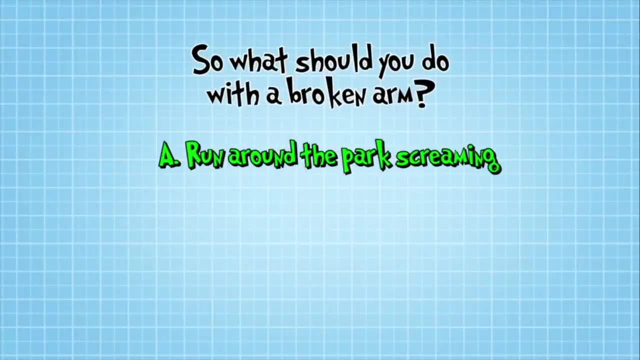 Sounds like an injury alert. So what should you do with a broken arm? Should you: A. run around the park screaming My arm's broken, B. support it to stop it moving, using your hand, some clothing or cushions, Or C. tell your teacher? 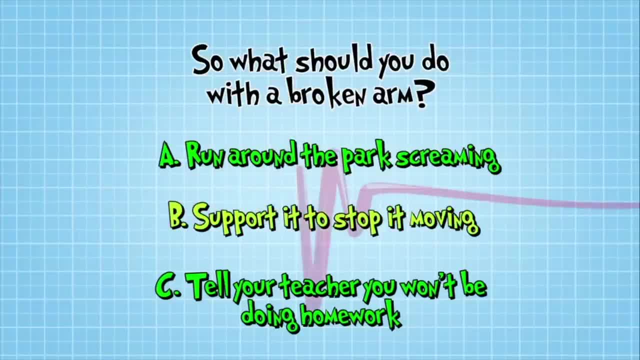 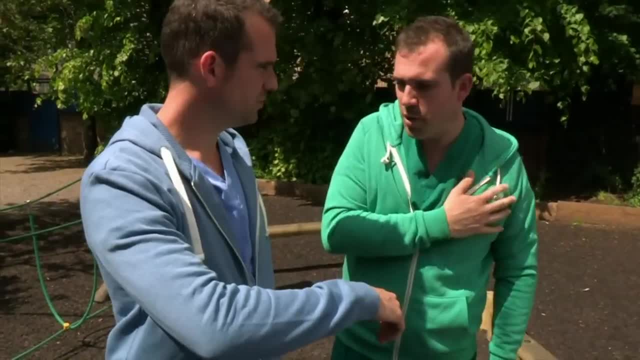 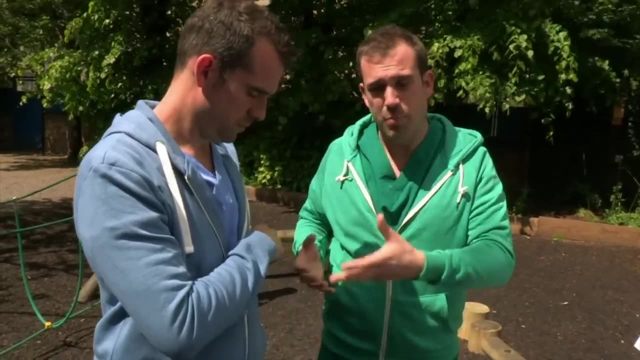 you won't be doing homework ever again. You guessed it. the answer is B. Here's how it's done. So, Chris, put your arm against your body gently as you can. It really hurts if I move it, And then what we can do is use Chris's jumper to support the arm itself. 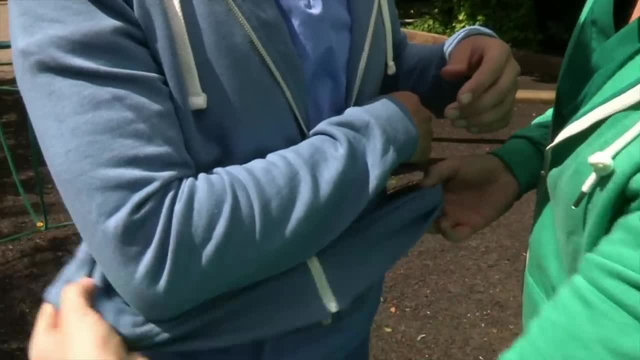 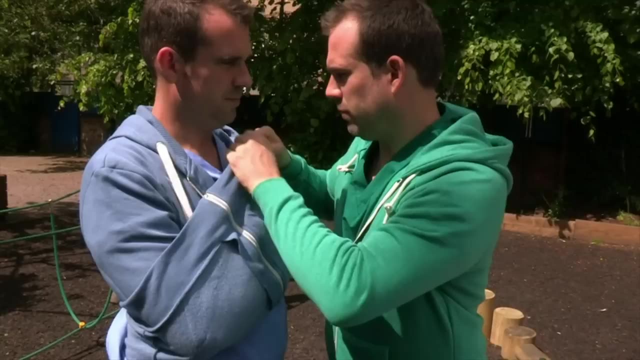 So we go very gently, try not to move the arm. Now, remember we're showing you what to do in an emergency. Never do this on your own, unless it is an emergency. Always try and find an adult. How's that? 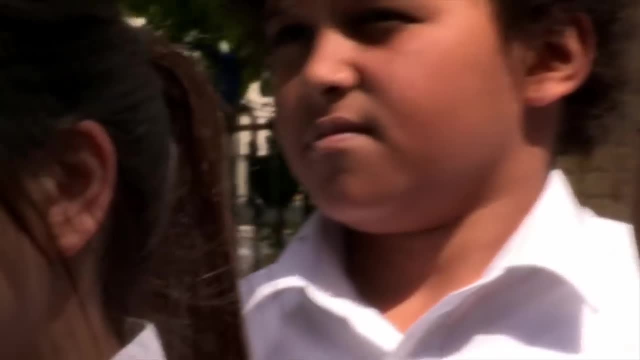 And can you now relax your arm? Yeah, that feels much better. Yeah, It's more comfortable, isn't it? So once he's feeling better, we can get him to hospital. He's going to be more comfortable when he's moving. 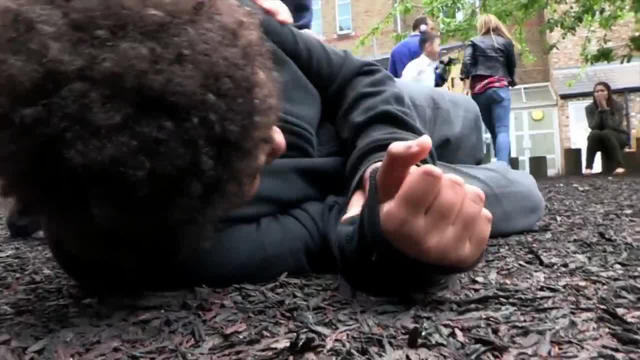 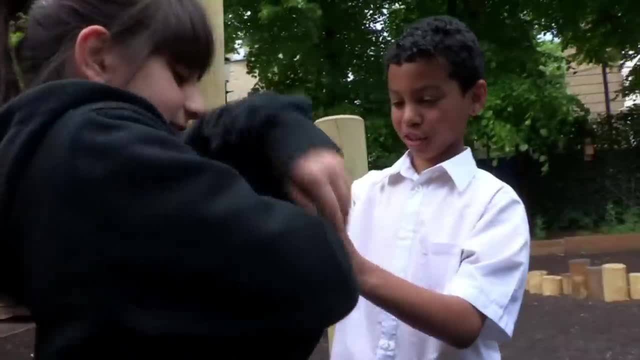 We can get him x-rayed and see what's going on. So now it's this lot's turn to have a go. That's really good. So try and be very gentle with that arm. How's that feeling? Can you relax that arm now? 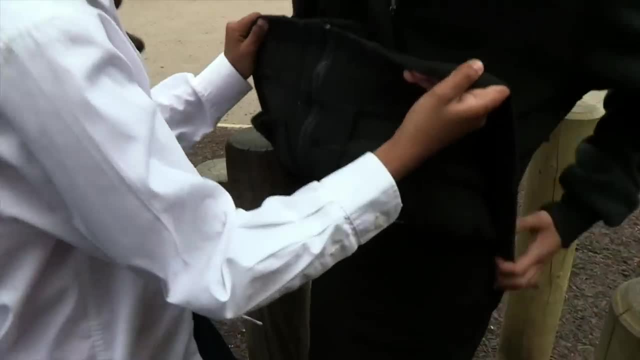 Feels pretty good. Yeah, it feels a little better. So obviously, for most of the time when you've got a broken arm, you don't need to call the doctor, You don't need to call an ambulance. You can get in a car and go to A&E yourself. 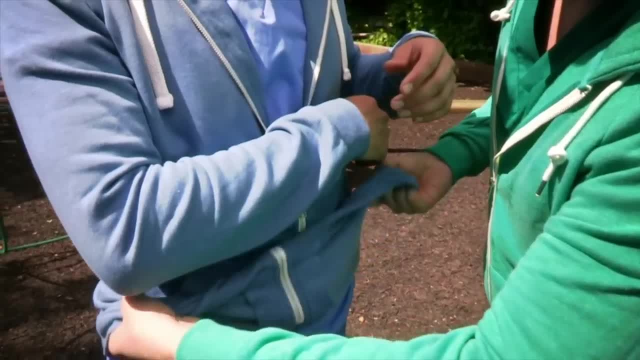 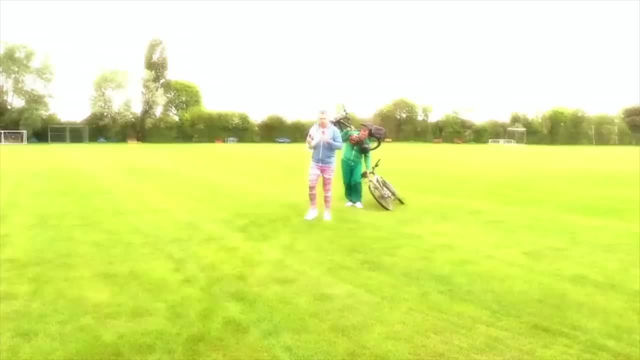 So if you think you might have broken your arm, support it to stop it moving using your hand or clothing or cushions, and tell an adult or call 999.. Are you sure it's broken, Chris? Better safe than sorry, Zahn. 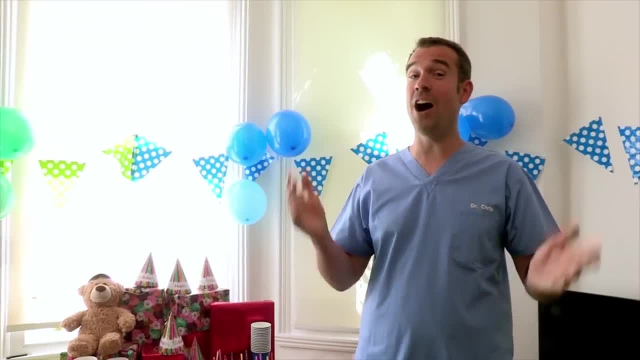 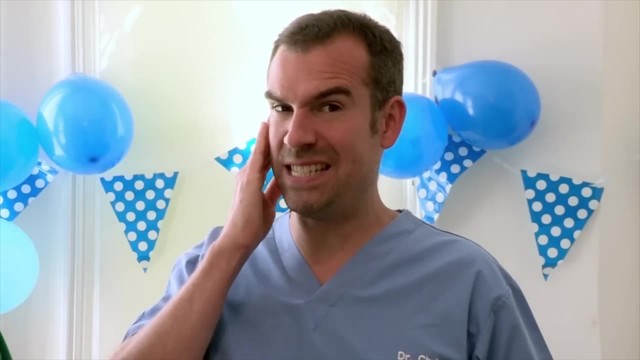 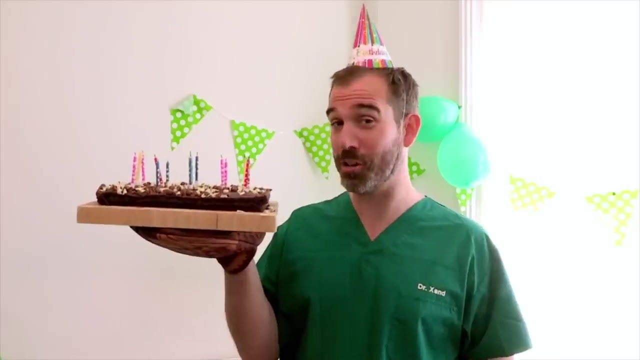 Today is a very exciting day for me. I'm going to get me and Dr Zahn because we're having our birthday party. As you can see, having a birthday party can be dangerous. You could burn yourself while you're baking the cake. 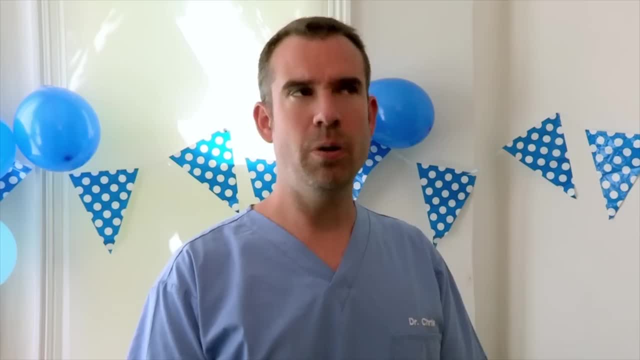 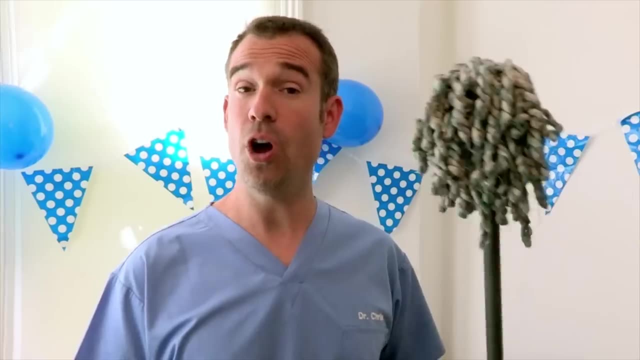 Not if you wear oven gloves or you buy it from the shop. Well, you could poke someone in the eye with the end of your party hat- Not if you're as careful as I am. Or you could slip on the freshly washed floor whilst practising your dance moves. 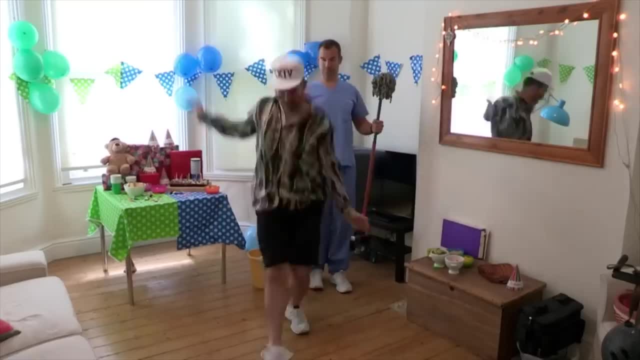 Or if you're in a hurry to go to work. Or if you're in a hurry to go to work, Or if you're in a hurry to go to work. Right, Zahn, come on, We've got to lay out the food for the guests. 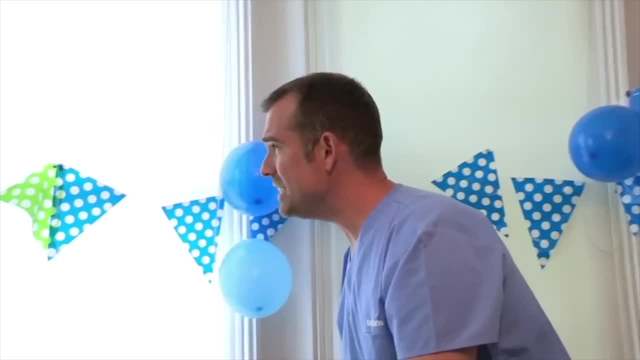 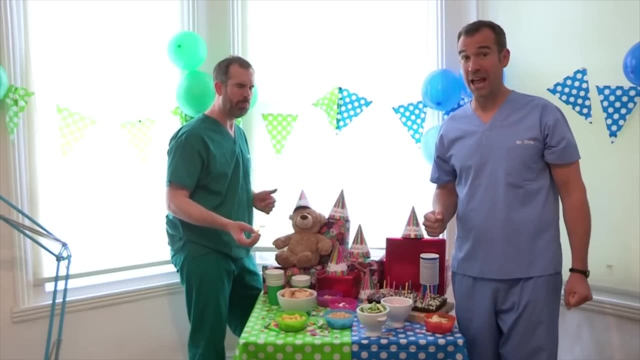 Ooh, don't mind if I do, And remember, don't eat anything from the bowl on the left. It's got peanuts in it and you can't eat peanuts. Zahn. This could cause a severe allergic reaction. 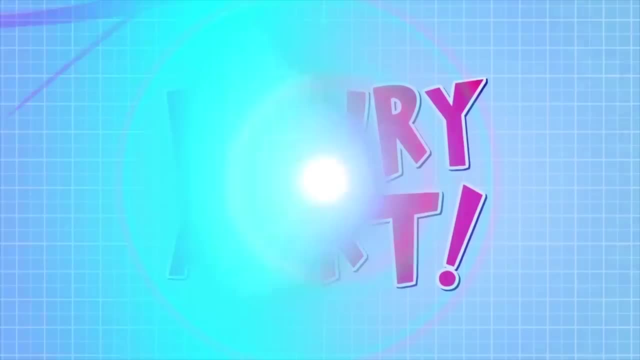 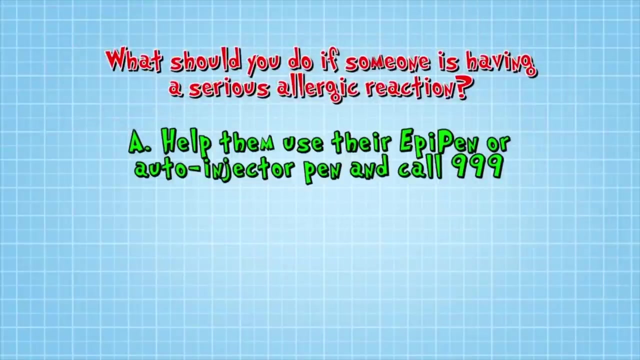 Injury alert. Now what should you do if someone was having a serious allergic reaction? A- Help them use their EpiPen or auto-injector pen and call 999.. B- Sing them a lullaby to help them feel calm. 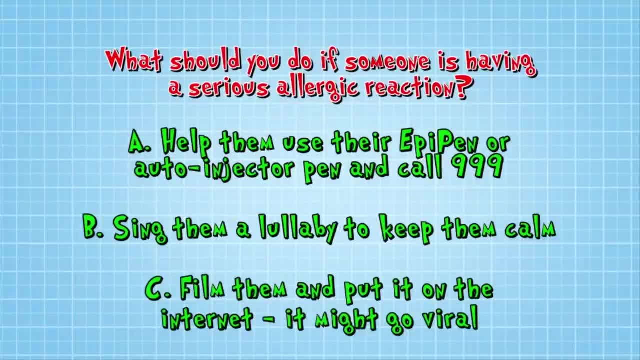 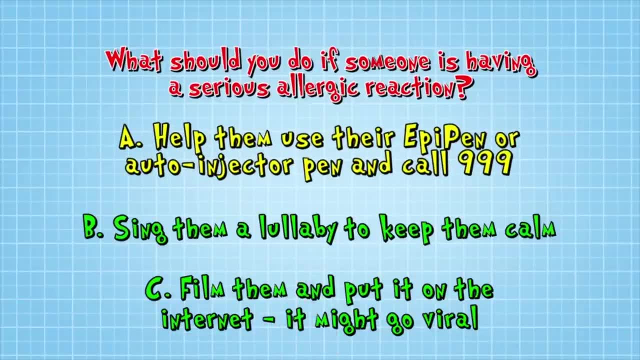 Or C- Film them and put it on the internet. It might go viral. The correct answer is: A- Help them use their EpiPen or auto-injector pen and call 999.. Let's see if this lot get it right without any help from us. 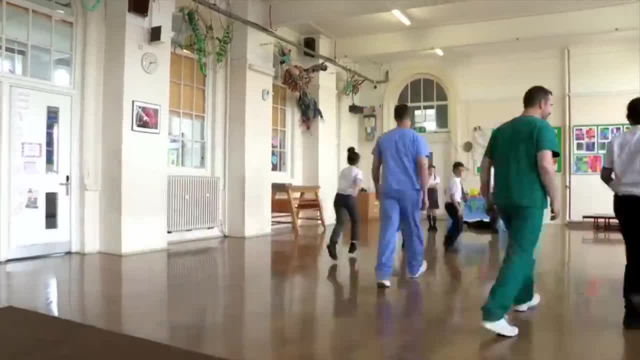 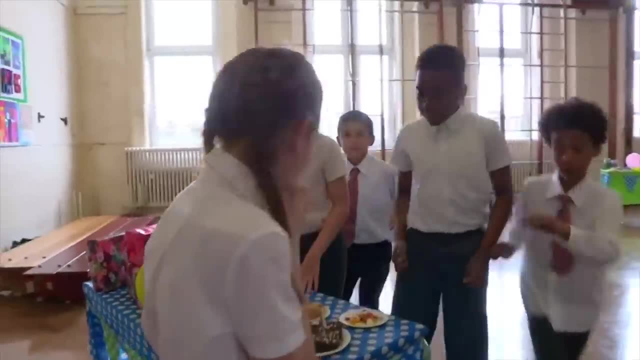 Right off you go. Ruby and Jessie are both pretending that they're having an allergic reaction. Quick, They need your help, Are you all right? Are you all right? Both teams get straight to work. I know, I'm just saying that I haven't eaten. 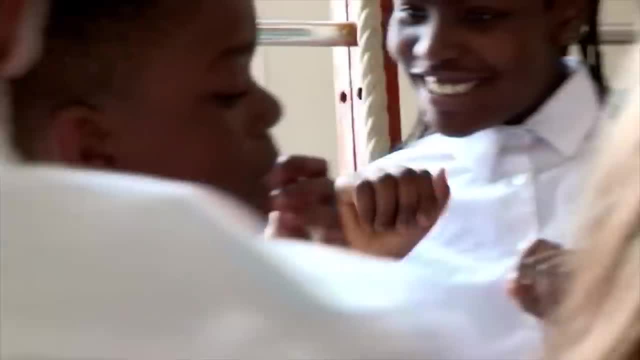 What happened to the peanuts? Quite rushed and quite panicked initially, I found this What They managed to find- the auto-injector pen. but they're stumbling a little bit with reading instructions properly. Our teams didn't quite get this right. They had some good ideas. 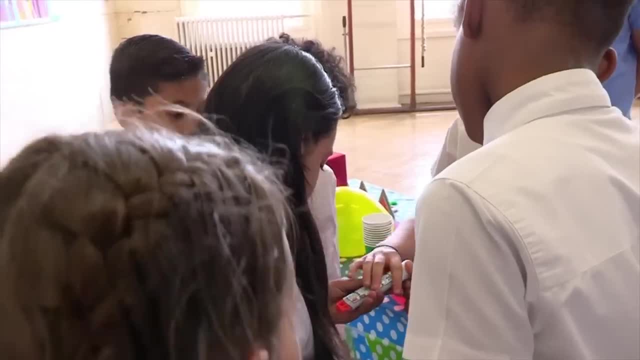 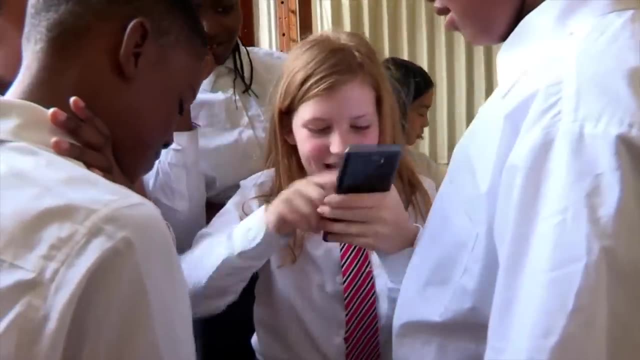 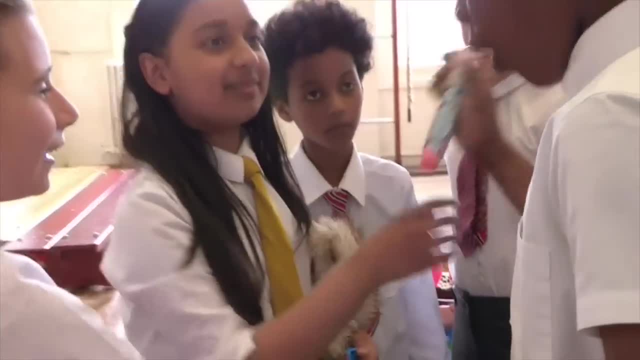 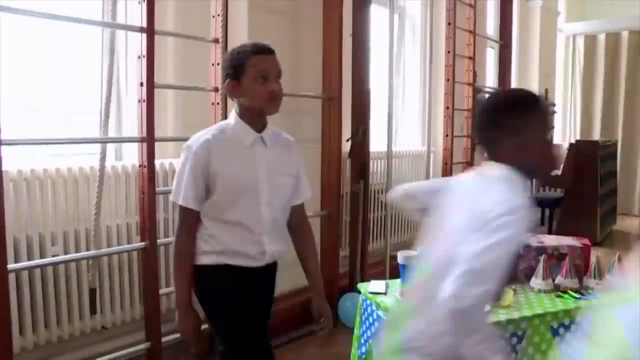 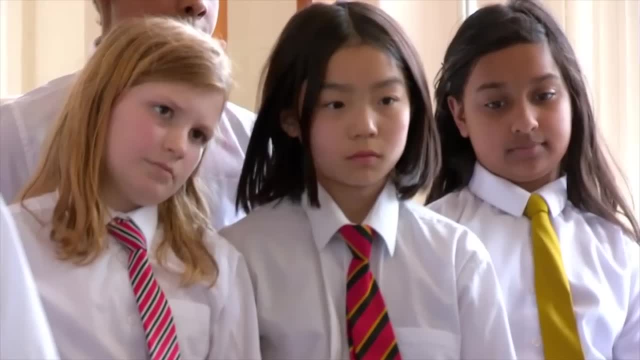 Come on, Remember, this is what to do in an emergency, but it's always best to get an adult. We're showing you what to do using a dummy injector pen. So let's say I'm having an allergic reaction, Chris, my lips are swelling, my tongue's swelling. 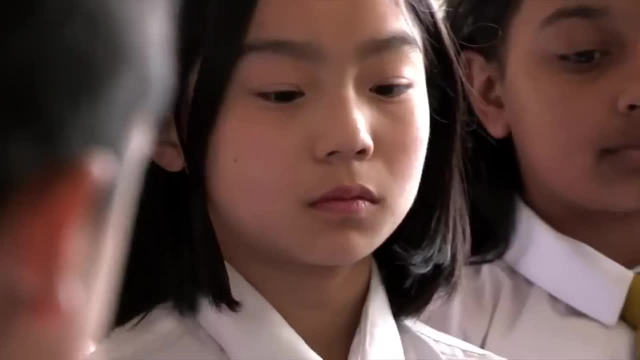 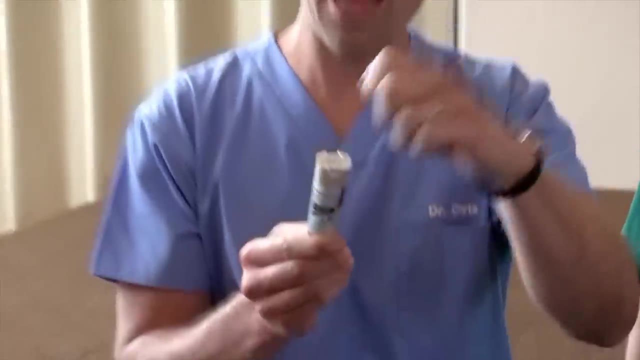 I'm feeling itchy in my mouth. I'm actually finding it quite hard to breathe now and I just feel terrible. I've got your auto-injector pen here, so I'd read the instructions. pull off the blue safety cap device 10 centimeters from the outer thigh. swing and jab orange tip firmly. 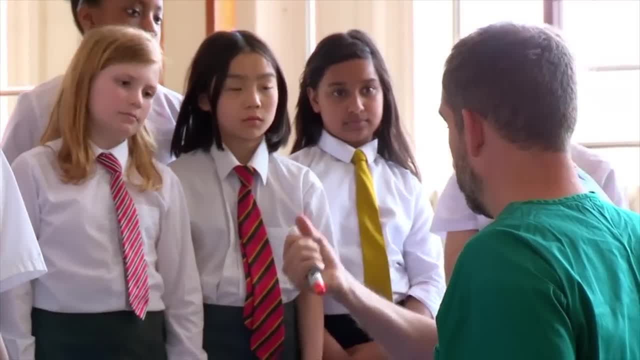 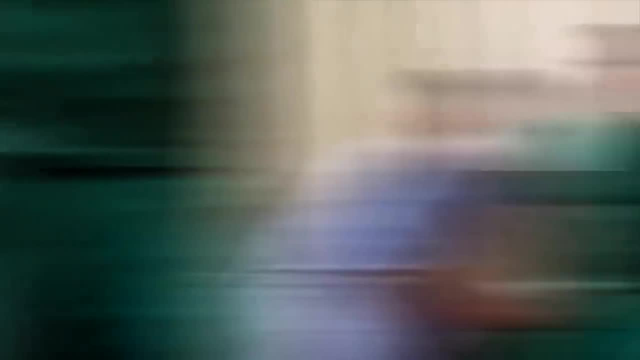 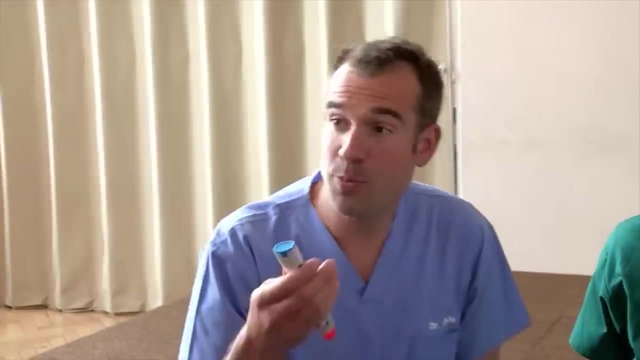 against outer thigh and listen for the click and hold in place for 10 seconds. so that's on to outer thigh. so that's about 10 centimeters. 1, 2, 9, 10, let me come out. and then it says massage area for 10 seconds. different pens have 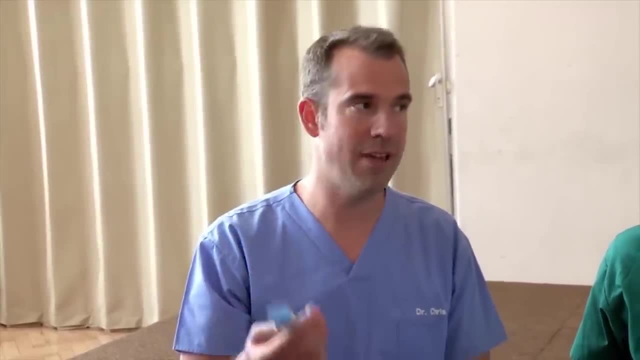 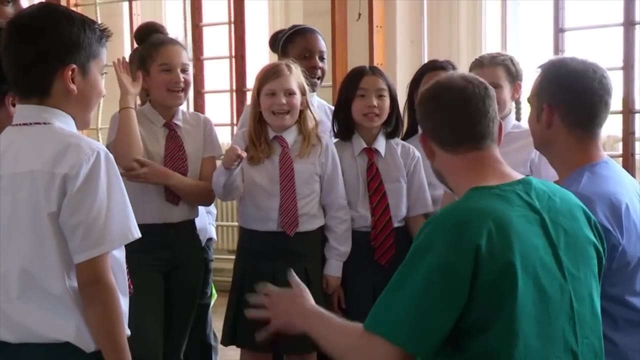 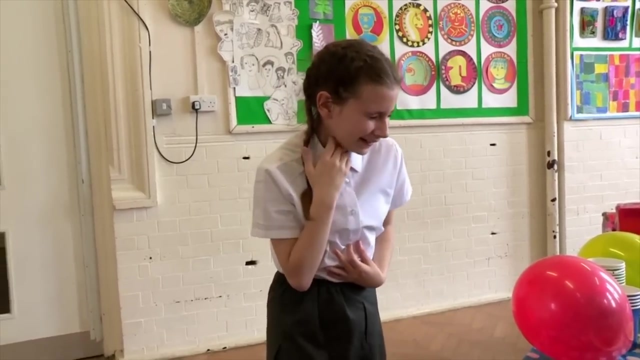 different sets of instructions, so always read the instructions carefully. once you've given the medicine, you must then call 999. right, who wants to try it again? come on then. so if you see someone with a rash, itchiness, swelling on their face or having difficulties breathing, then it might be a severe allergic reaction. and 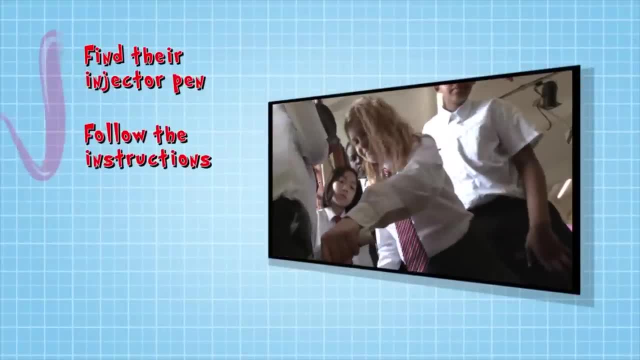 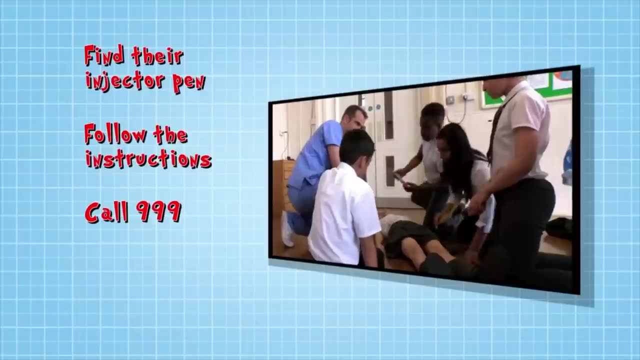 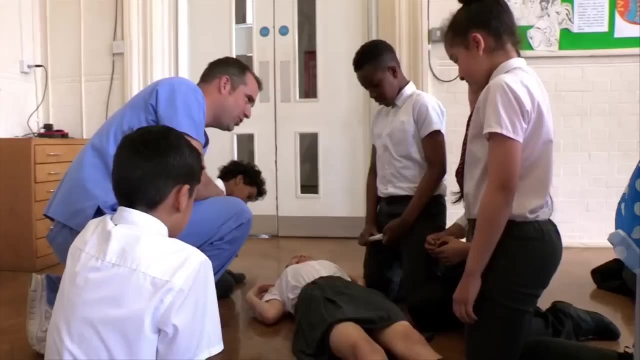 you must find their auto injector pen and help them to use it. following the instructions, call 999 and remember to find out your location. reassure the patient until the paramedics arrive and if they don't have an auto injector pen, call 999 immediately. really good job. 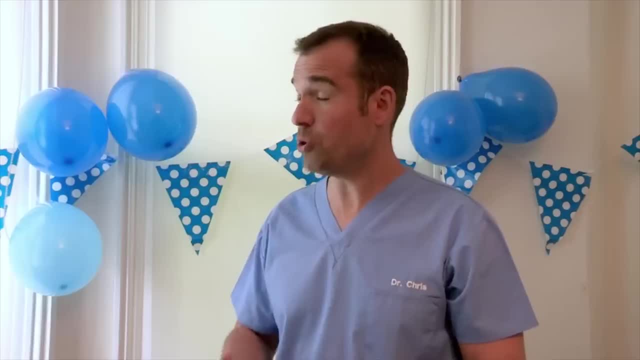 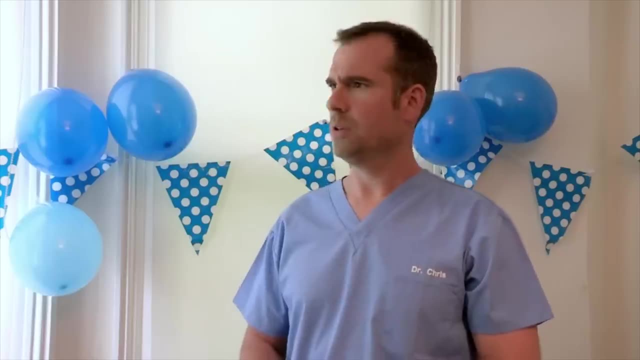 everyone. so are you okay? is your tongue itchy? is your throat swelling up? I can get your auto injector pen. I don't need my auto injector pen. yeah, you do. don't be silly, I didn't eat any peanuts, just been eating these sweets, although I see. 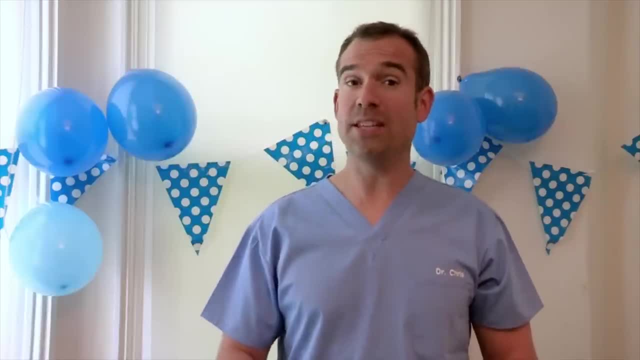 what you mean. they do look a bit similar. well, that is a relief, but it's always better to check if someone needs your help and if you have a friend or a twin brother with a severe nut allergy, it's better not to serve any nuts at all. 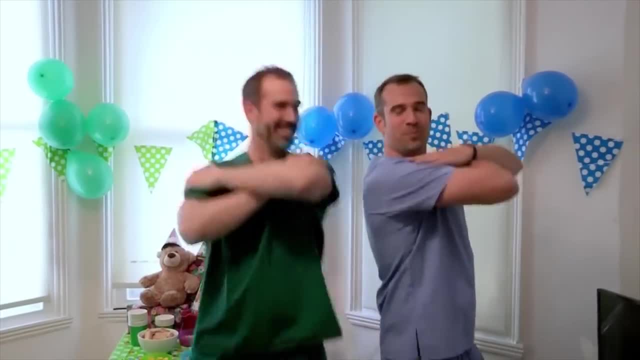 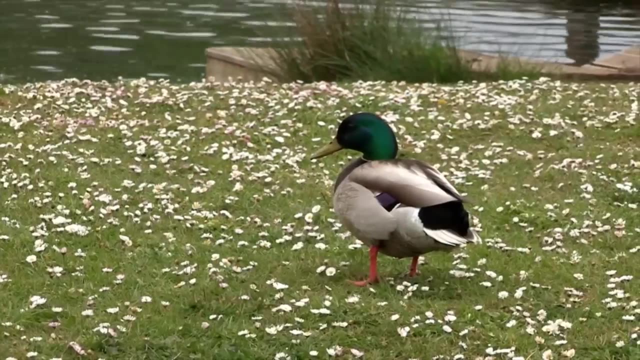 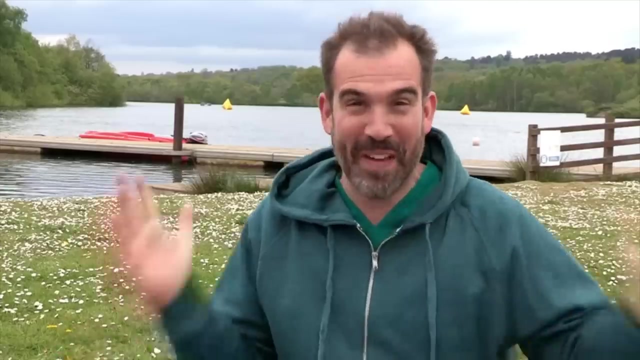 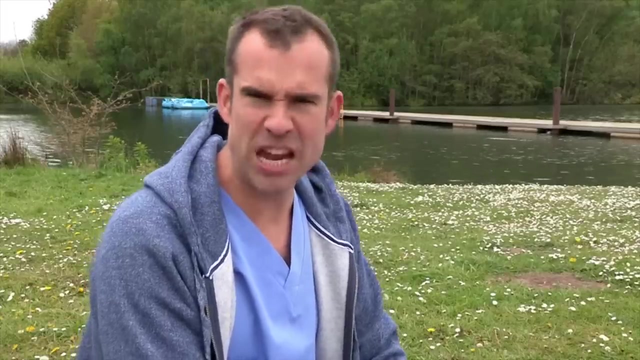 having a day out in the park or countryside is a brilliant way of getting some fresh air and chilling out. especially well, there's somewhere to swim. this defined by hvorom the belt. for some reason, UK, he did not pay for crips, but he외 to swim. 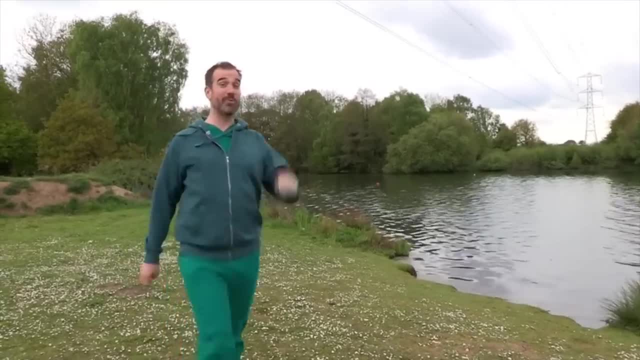 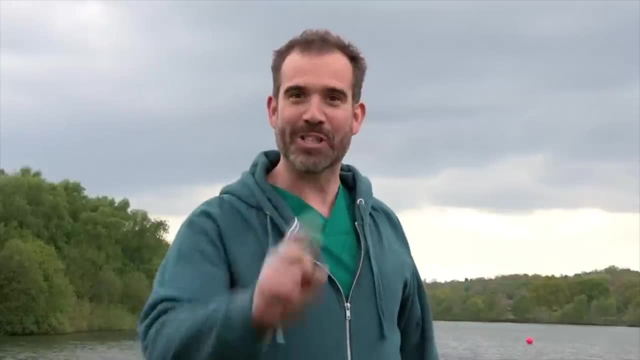 oohah, oh, not me. I always walk slowly and safely to the water's edge. well, you could get into a tangle trying to change into your swimming trunks and fall over, not if you've already come wearing your swimmers under your clothes. well, you could stub your toe on rocks getting. 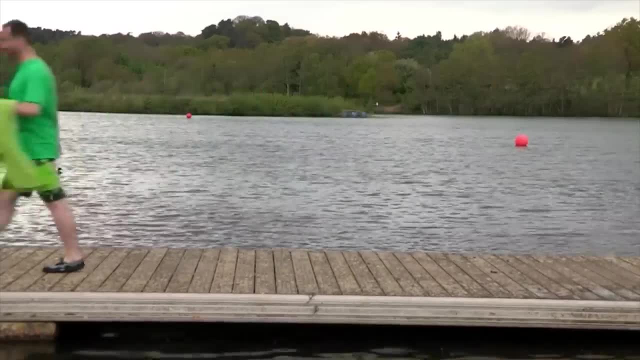 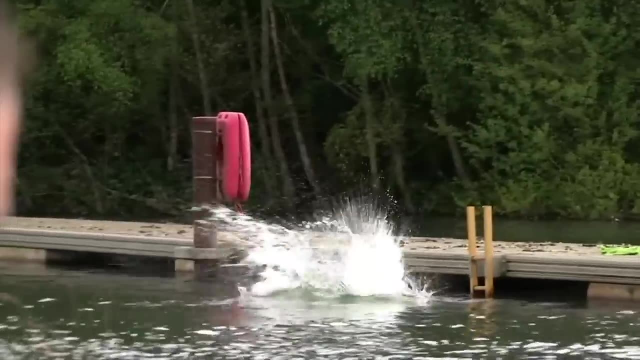 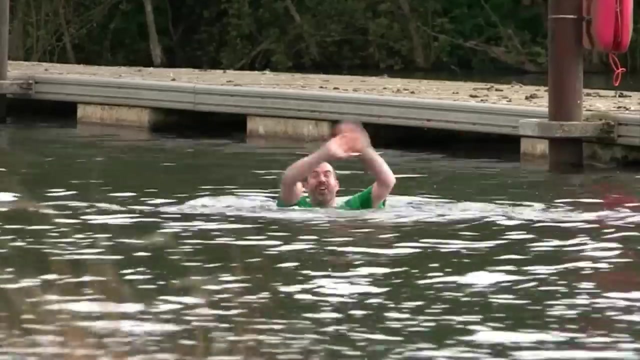 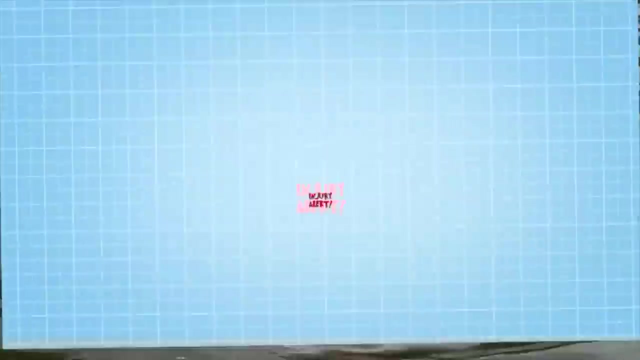 into the water, not if you use the jetty, Chris. well, in that case I needn't have worried. I'll just sit back and read my book. this looks like an injury alert. I better save him. if you see someone drowning, never jump in to rescue. go and get an adult once they've been rescued from the. 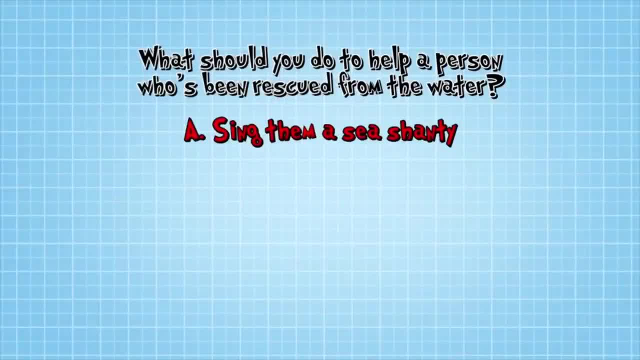 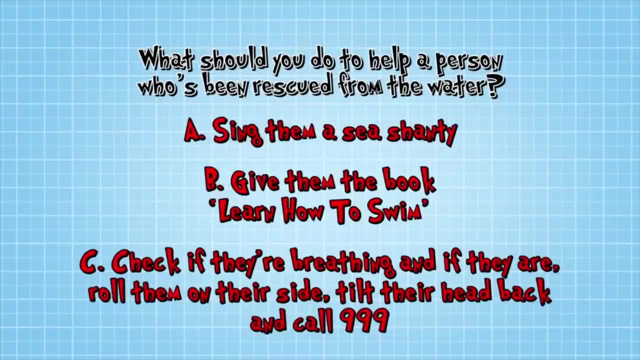 water. should you: a- sing them a sea shanty, B- give them the book learn how to swim. and Or- C- check if they're breathing and if they are, roll them on their side, tilt their head back and call 999.. The correct answer is, of course, C- check if they're breathing. 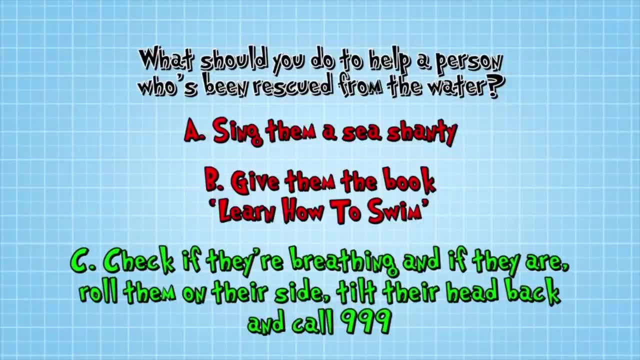 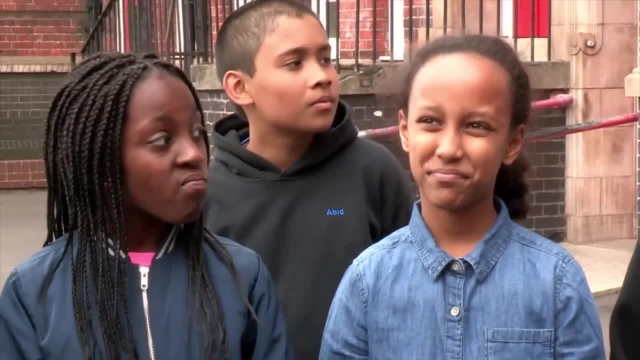 and if they are, roll them on their side, tilt their head back and call 999.. Let's see if this lot get it right. They've not had any advice and they're winging it. Are you ready? Yeah, Off you go. 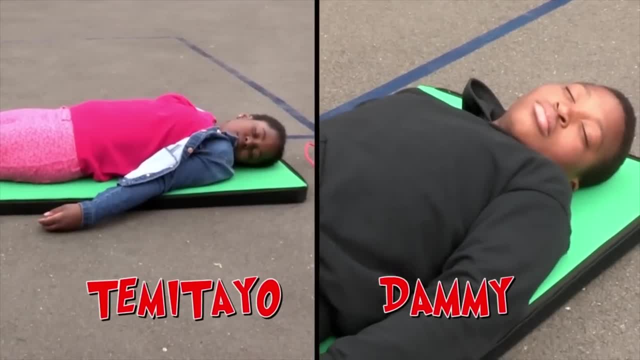 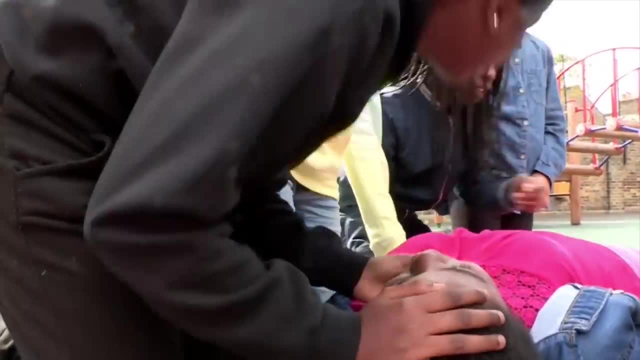 Temetayo and Dami are both pretending that they've been rescued from a lake after they started drowning. Quick guys, they need your help. Is she breathing? Yeah, she's breathing. Checking she's breathing is a great start. I'll maybe try and start doing chest compressions. 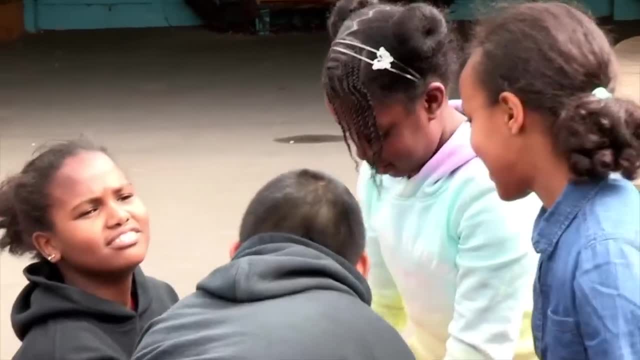 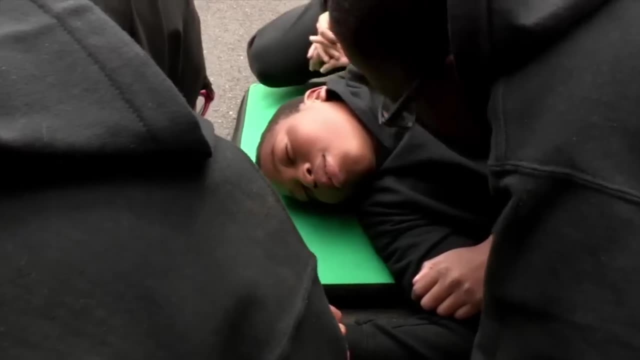 They know she's breathing and they're still doing chest compressions, which isn't going to do any good at all. We're going to put him on his side. They put him on his side, but they didn't check anything first. How do you get water off someone? 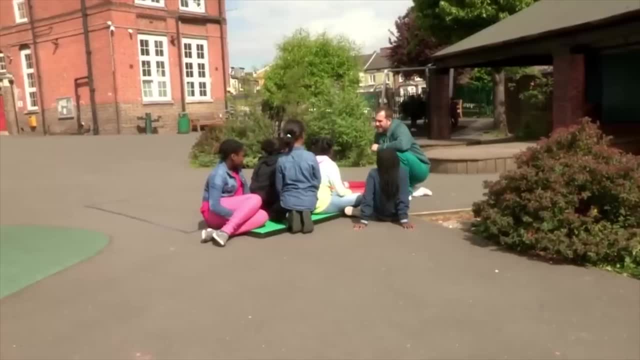 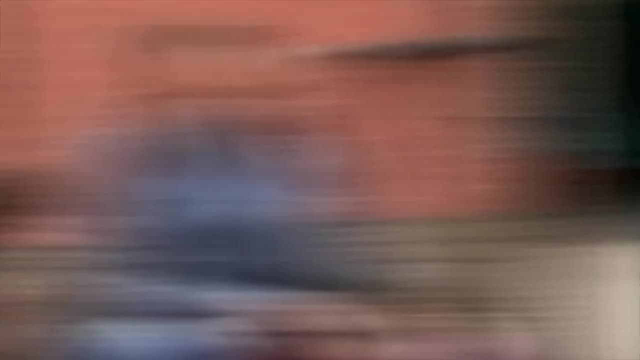 They haven't worked out if he's breathing or not. OK, Our teams didn't quite get this right. They had some good ideas. I put him into the rescue position and a few dodgy ones. Mirabelle, why did you start doing chest compressions? 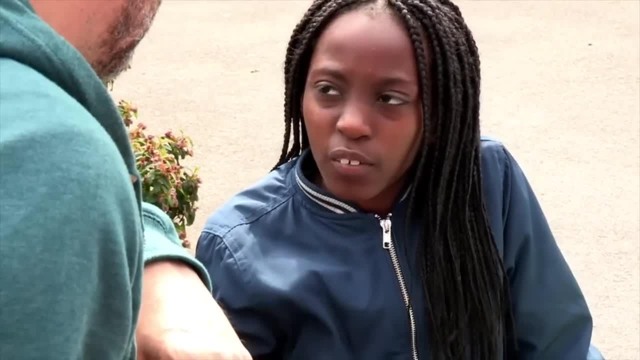 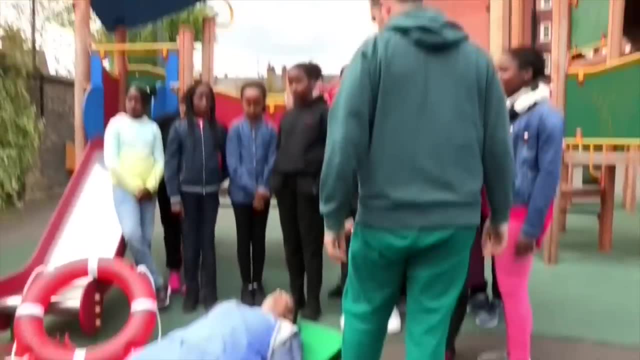 Just so that she can at least get a bit of water out of her system. So you were trying to squeeze her out like a sponge Time to show you how it should be done. So Chris just been pulled out of the lake, but he's not responsive. 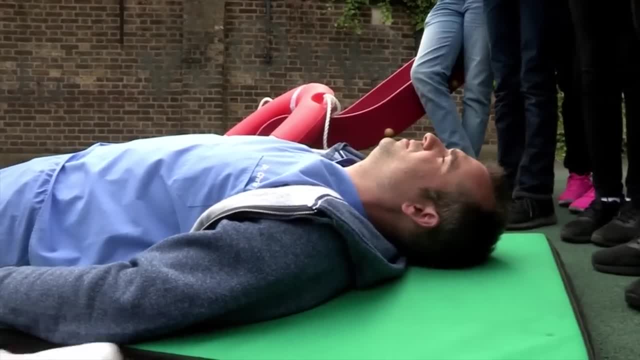 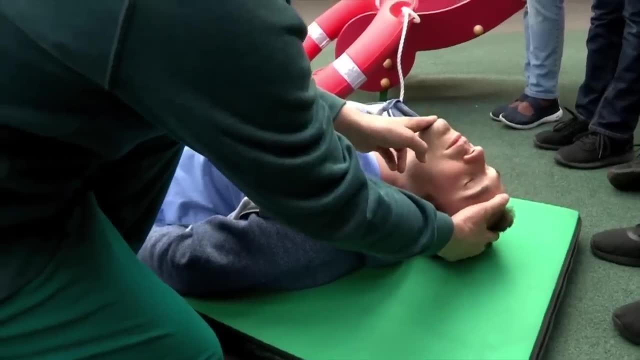 Remember, we're showing you what to do in an emergency, but it's always best to get an adult After you've checked he's unresponsive, check that he's breathing, So I'm going to tilt his head back, his mouth open. 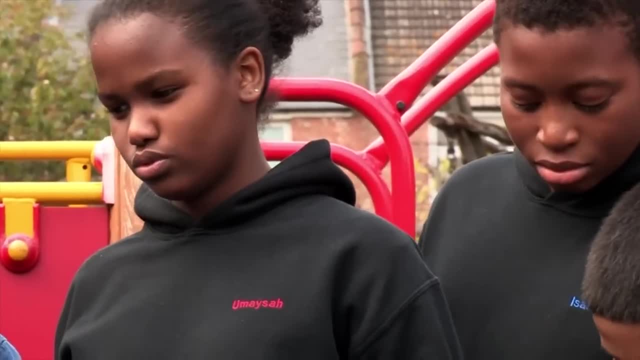 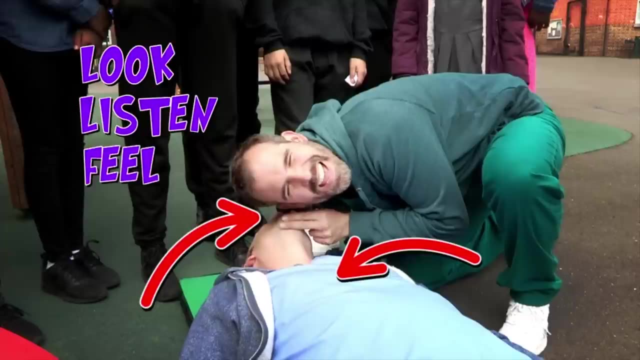 To work out. if someone's breathing, place your face close to theirs, Look, Is their chest moving, Listen, Can you hear them breathing And feel. Can you feel their breath on your face? And he is breathing, but he's not responsive. 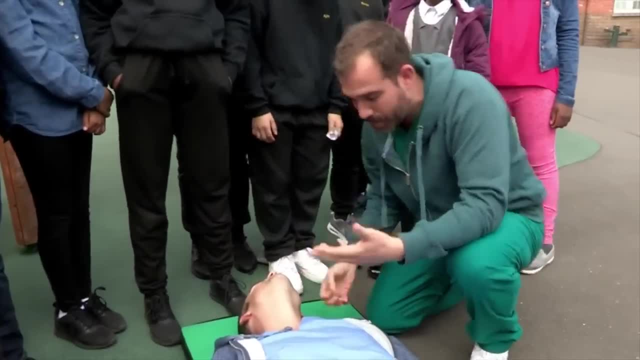 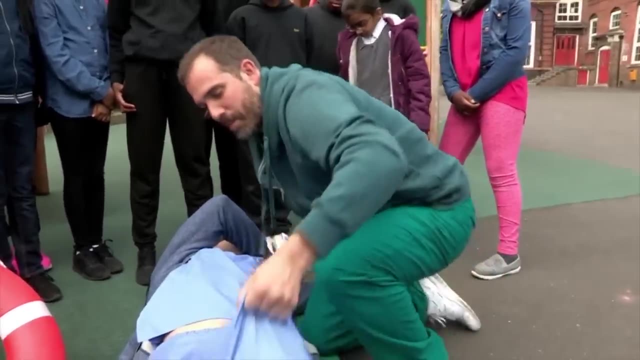 So the next thing I need to do is get him in a position which will keep his airway open. Get that arm up, This arm over here, This leg up, And roll him towards me. Most important bit is to tilt his head like that. 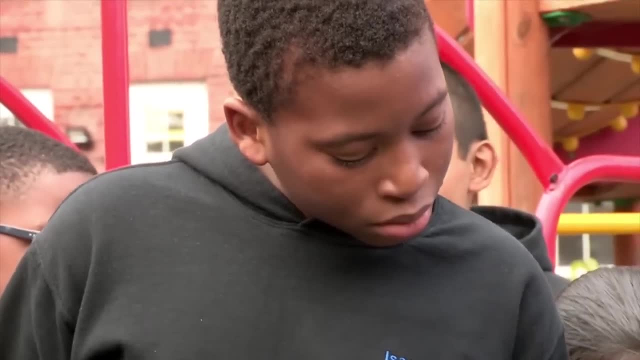 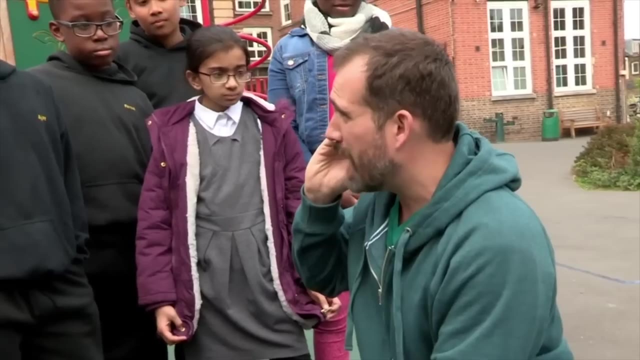 so that his airway is open. This also helps any water come out. And now I phone the ambulance, 999.. Give my location, Say what's happened, Say that I want an ambulance And they'll be on their way. While you're waiting, keep checking. the person is still breathing. 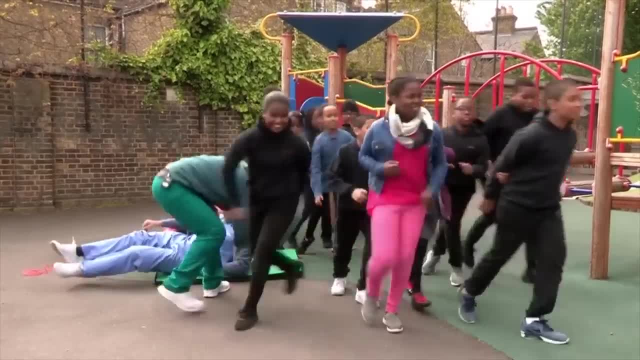 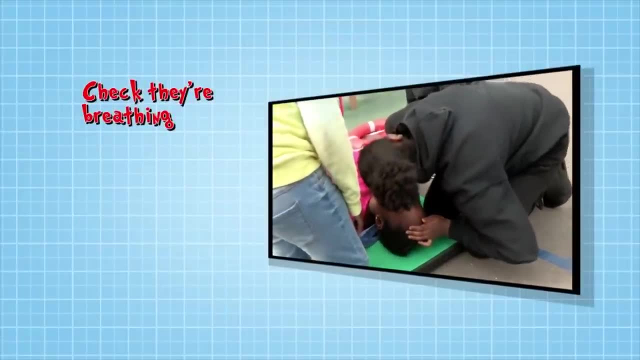 Are you ready to have another go? Yeah, Off you go. So if you see someone who's been rescued from drowning and is unresponsive, check their breathing And if they are, roll them onto their side, tilt their head back and then call 999.. 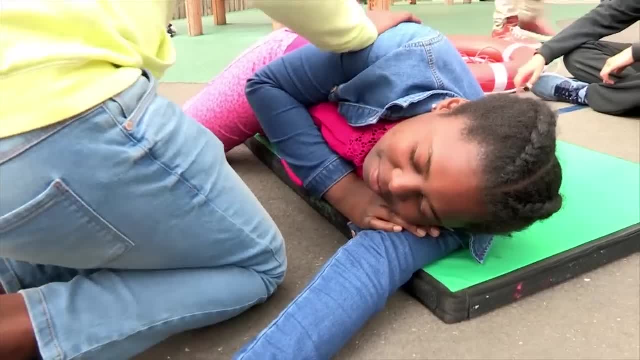 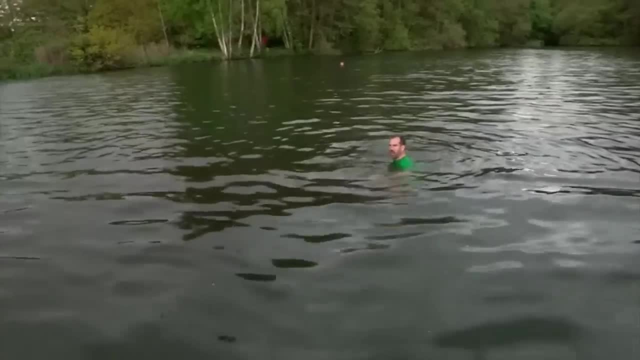 He's breathing, but she isn't responding. If the person isn't breathing, the response is different. You must call 999 immediately and find an adult. Don't worry, son, I've got you. I'm not drowning. I was waving to say hello. 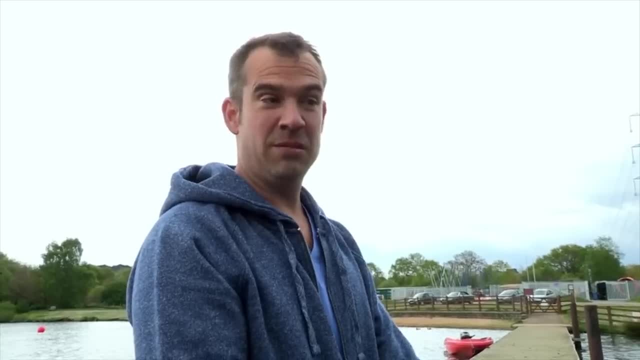 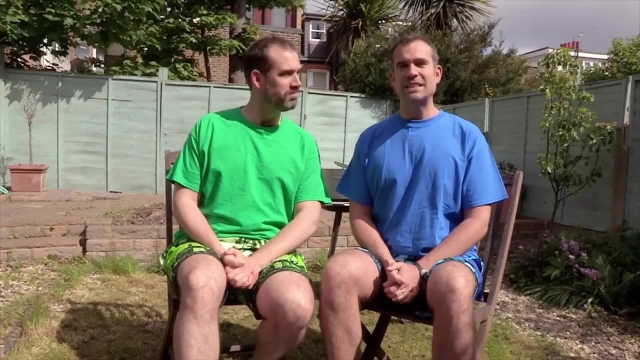 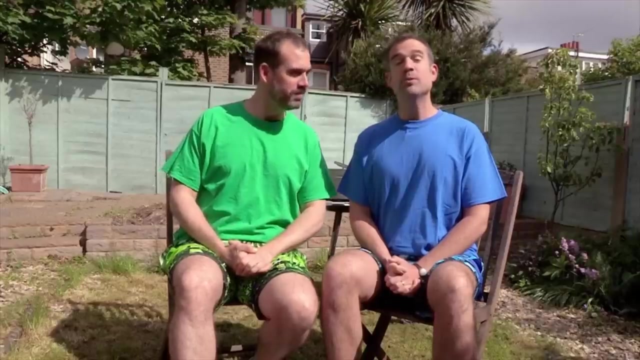 Oh well, always better to be safe than sorry, I say One of Zahn and my favourite activities in the summer is to have a barbecue, And today we're having my favourite sausages. But remember a barbecue in the garden. 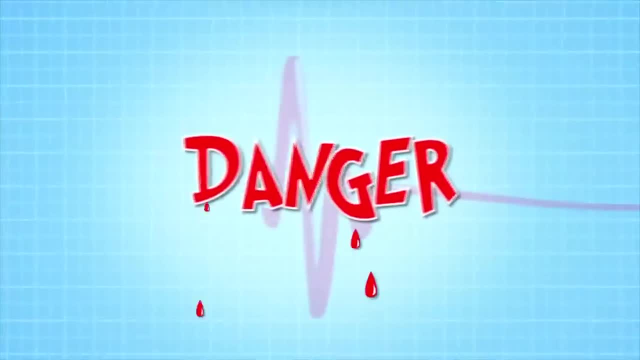 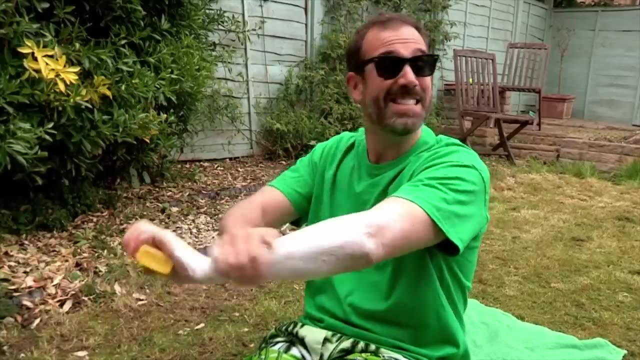 can also be full of potential danger. Don't stay out in the sun too long or you could get burned. Not a worry for me, Chris. I never use anything less than Factor 30.. All right, well, be careful when you're playing ball games. 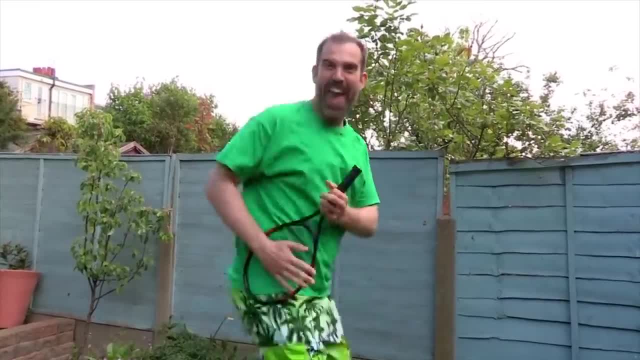 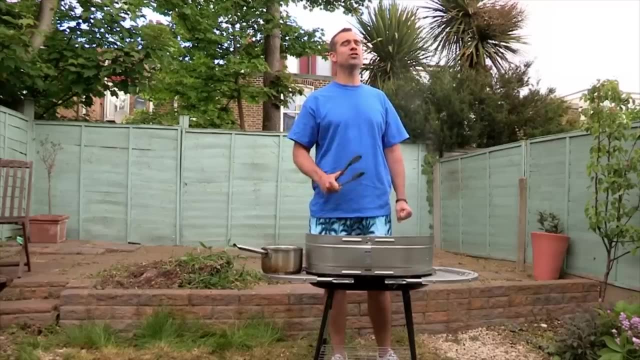 where you could hit someone on the head, Not if you only use it for air guitar. Well, in that case we can get on and enjoy the barbecue. Zahn food's ready sausages and piping hot beans. Ah, My leg. The piping hot beans have burnt my leg. 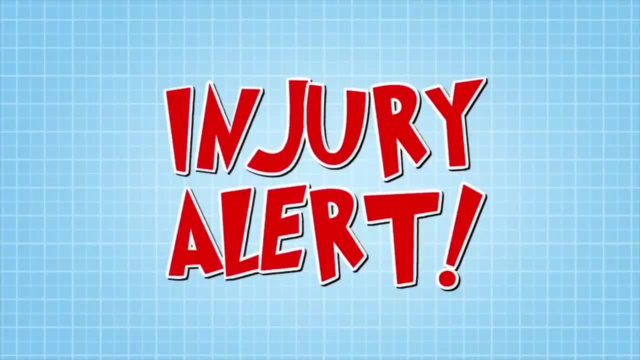 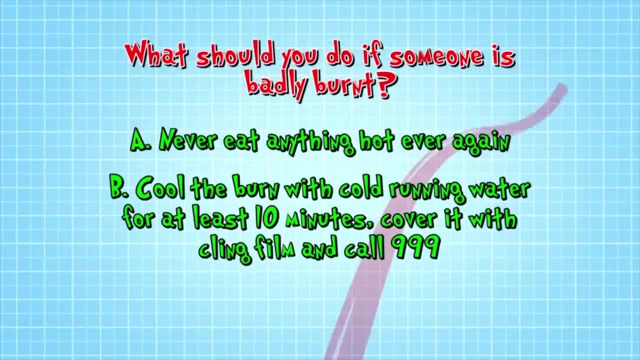 Injury alert. What should you do if someone is badly burned? A- never eat anything hot ever again. B- cool the burn with cold running water for at least ten minutes, then cover it with cling film and call 999.. Or C- shout out if you can't stand the heat. 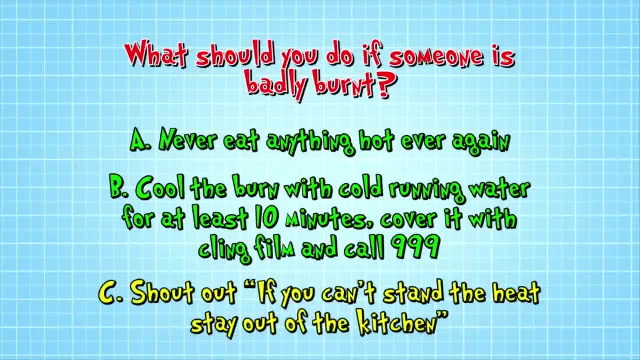 stay out of the kitchen. Well, the correct answer is: B Cool the burn with cold running water for at least ten minutes, then cover it with cling film and call 999.. Let's see if this lot get it right. They've not had any advice, so they're winging it. 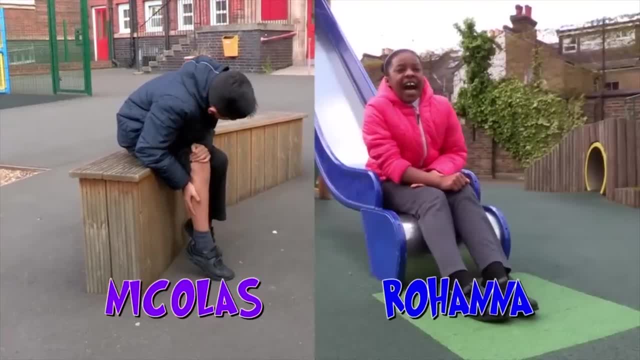 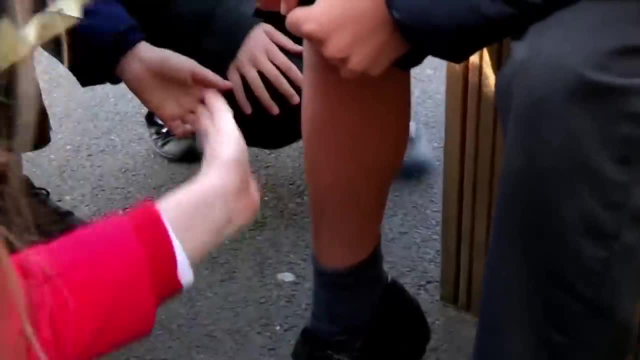 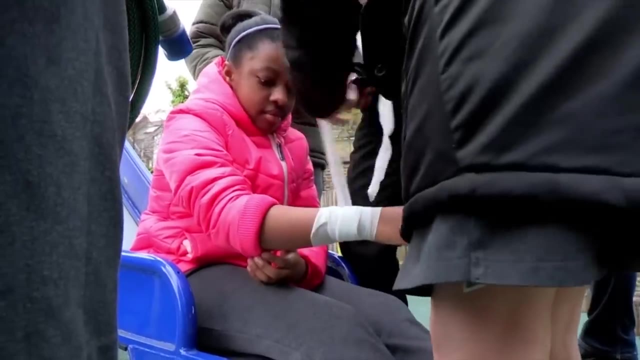 Go. Nicholas and Rohanna are both pretending that they've been badly burned. Quick, everyone, they need your help. OK, let's go. They've used alcohol gel, which would be very painful if you had a burn. They're putting on a gauze bandage right onto the burn. 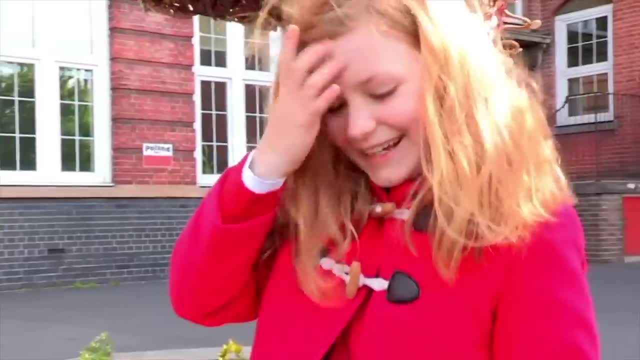 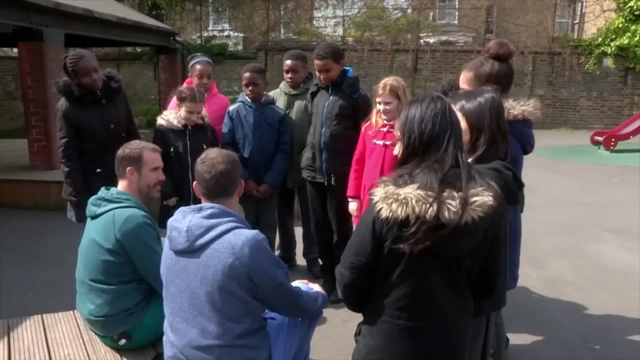 Not a good idea. on a severe burn, You have to take a picture. They've thought of using the phone, but unfortunately they've used the phone to take a selfie. OK, done, Time to show you how it should be done. Ah Ow, It hurts, I've burned myself. 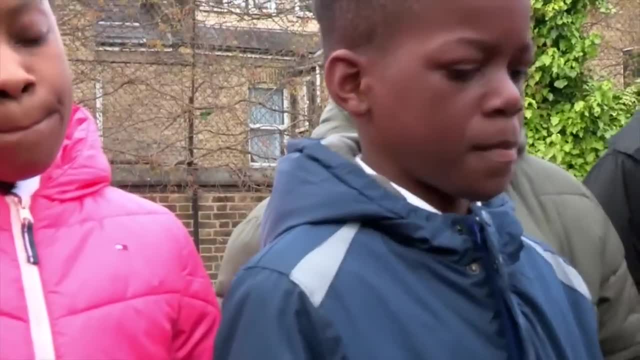 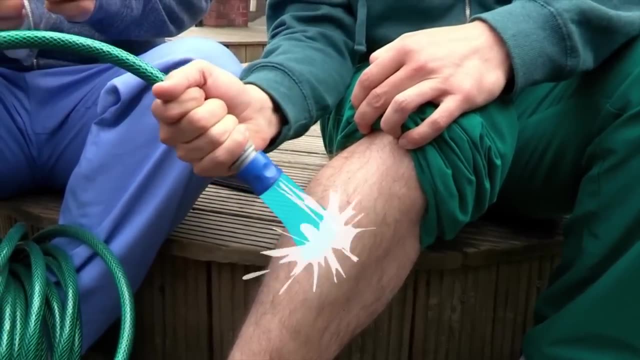 Remember, we're showing you what to do in an emergency, but it's always best to get an adult. Don't worry, Zand, it's all going to be fine. We pour cold running water over it for ten minutes using a hose like this. 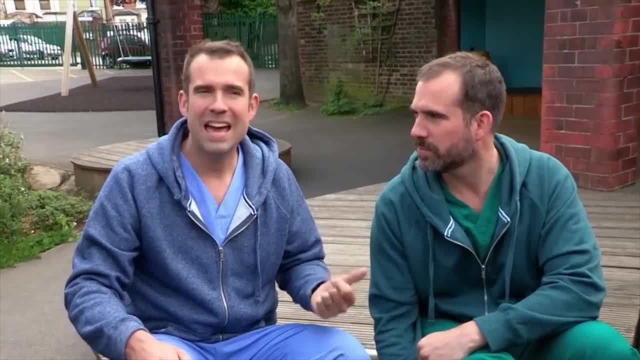 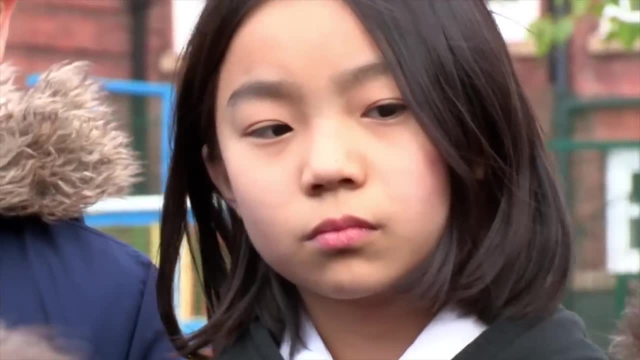 That is the most important thing you can do, because it reduces the temperature and it reduces scarring. So we do need to get Zand to hospital and a good way of doing that is by calling 999.. After ten minutes of cold water. 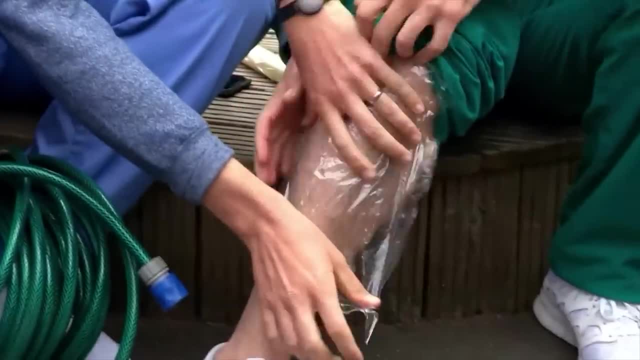 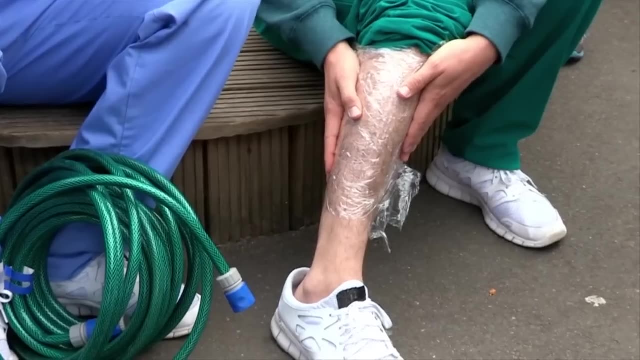 we then want to put cling film on and put it on the burn like that. So when you get a bad burn, you lose the top layer of skin, and that means you're at risk of infection, and so cling film acts like temporary skin.